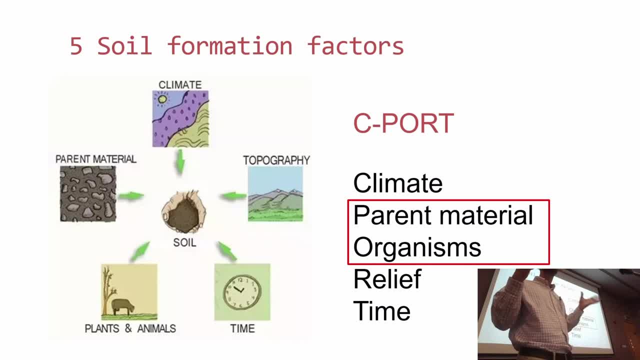 also how that rock was physically weathered, transported, sedimented and then developed the soil and then it was transported, and then it was transported, and then it was transported, and then the soil is important for you to understand the properties of that soil. so parent materials- not always most of the time they are transported before they are allowed to form the soils, okay, 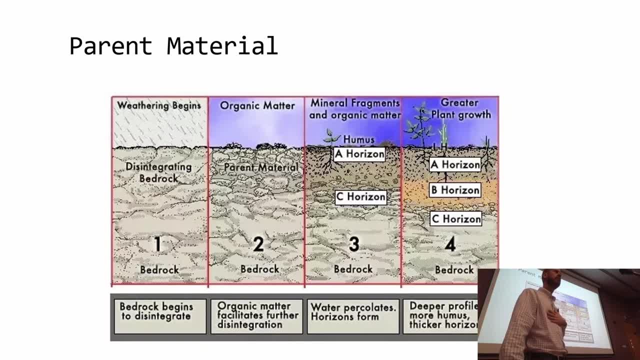 so in an ideal condition, textbook condition, you have the soil which is disintegrating over time and forming the soil in situ- yeah, forming the soil in situ- and there is the development of soil Horizons. how many of you heard about soil Horizons, the concept of soil Horizons? okay, a Horizon B Horizon, C Horizon. so a Horizon is. 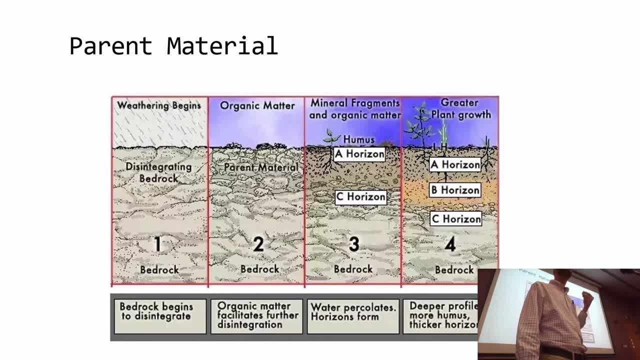 the, what we call the topsoil. okay, topsoil means that the ones that are being transformed by organisms and are very appropriate for sustaining the growth of plants. C Horizon is the one that is very similar to the original rock, the parent material. it's just fragmented, it's a regulate. yeah, in geological terms is the regular. 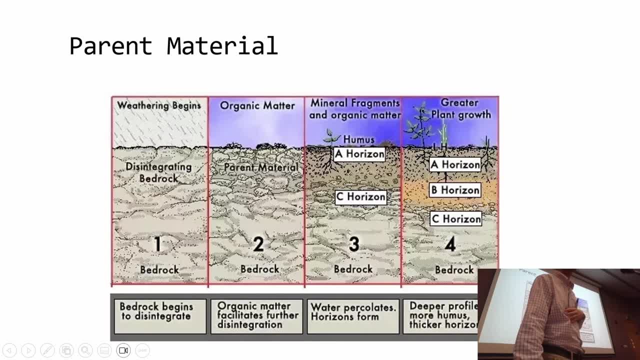 B. Horizon develops when you have mature soils is where it's a layer where there is deposit of some materials. yeah, the big Horizon will have some deposits. so when you see a big Horizon, that is accumulation layer in the soil is already a symptom that your soils are becoming mature. 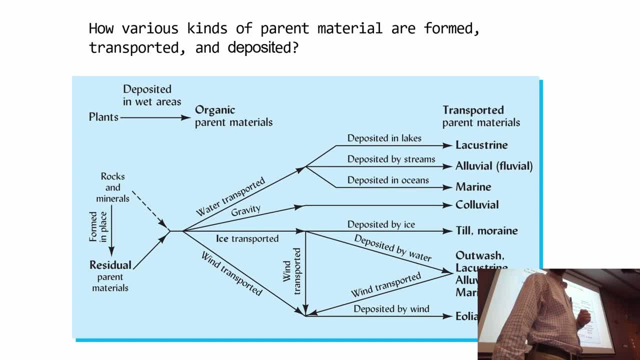 over time. so so residual parent material can be transported by different ways. so what are the ways that, based on this figure, how many different ways can you see them depending on each framework you wish? toảo koei, toa koe reviewed. based on this figure, how many different ways can you see them? 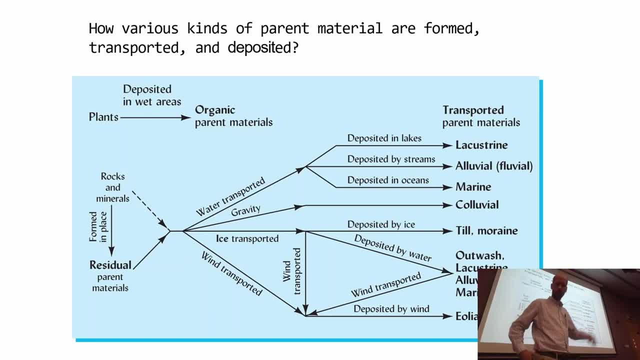 that the materials can be transported. so here is the agent of transportation. okay, how is the agent of transportation? so can be water transported, and depending of the type of water that is transporting, you have different names. if it's water transported. if it's deposit in lakes, it's lack of stream. if deposit. 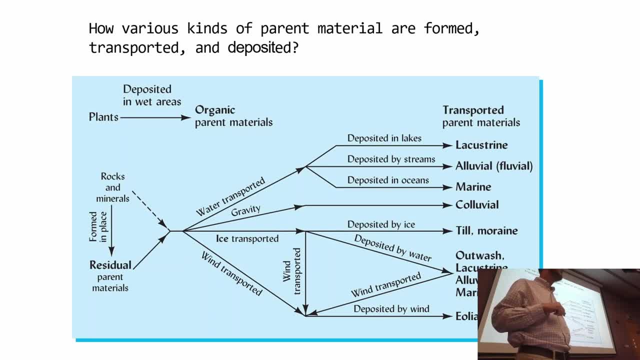 by streams is alluvial or fluvial. normally the name is alluvial. soils okay. deposit in oceans, marine- okay. now, if it's gravity, it's colluvial. how can gravity deposit materials? have you heard about landslides? yeah, landslides. have you seen that before? maybe, if you can just search. 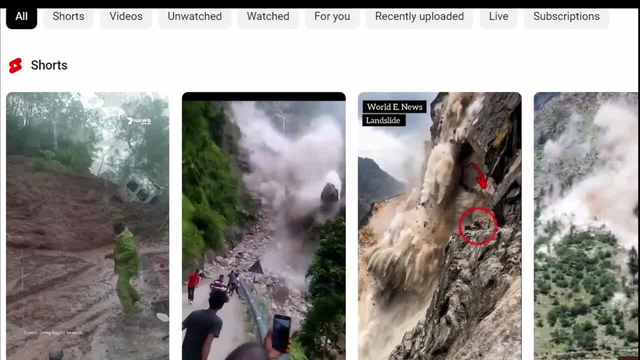 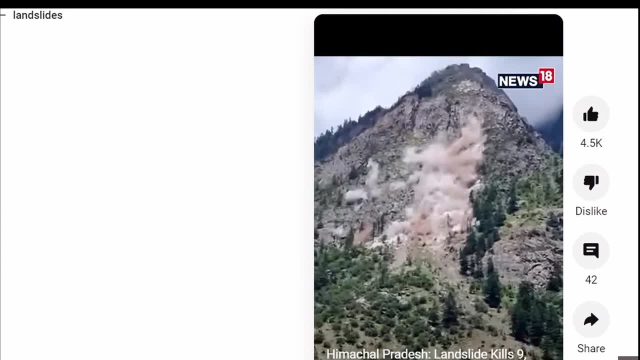 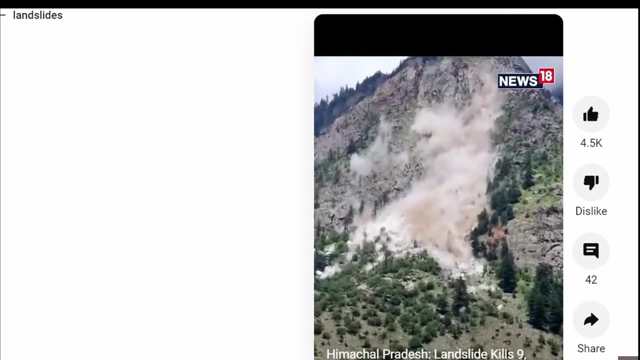 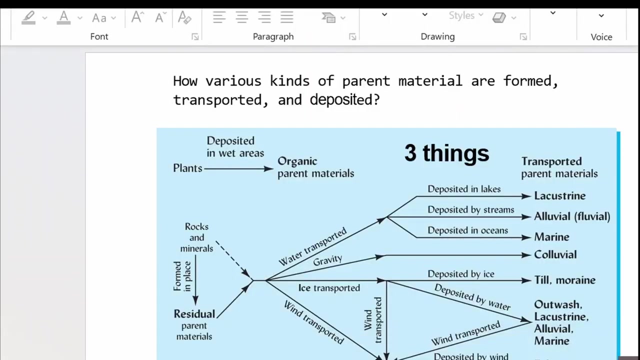 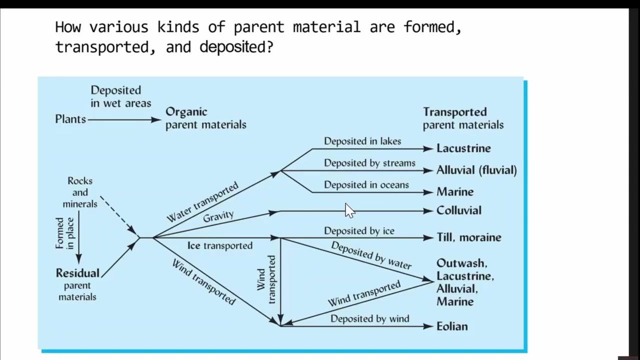 quickly here. other here of landslides: yeah, similar to an avalanche of snow, but only from rocks and mud and soil material. all right. so we have gravity making colluvial deposits, yeah, colluvial deposits. if it's ice transported, we call it till and moraine. yeah, and then if 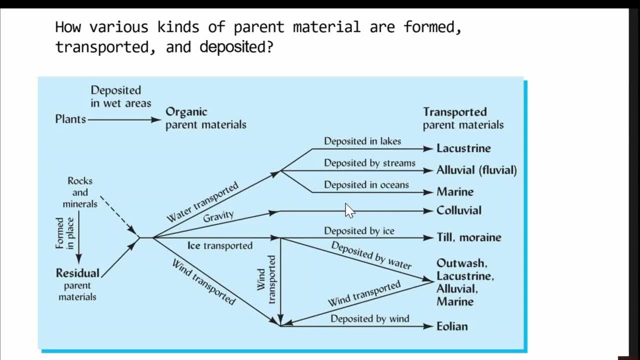 it's deposited by water, you have outwash, lack of stream, alluvial and marine again over here. how is it formed? because with the glaciers are pushing that soil around, we're going to come to this on the next slide. it forms a small features like small hills. it's pushing the soil around and 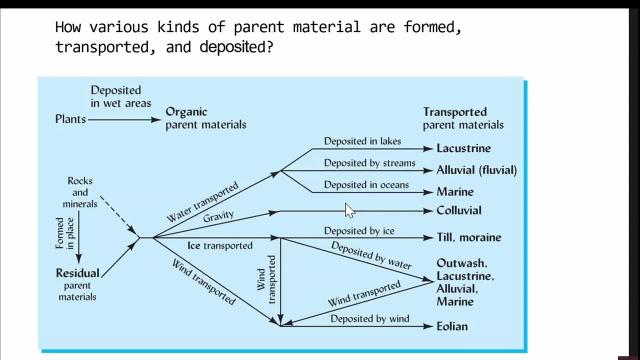 this is at the formations. that is the soil that's pushed around. but also when you have those glaciers, you form lagoons, yeah lakes about where. with that where, in that type of landscape, and sometimes that lakes, they break and they deposit the water further below. so it becomes, if it's becoming transported- 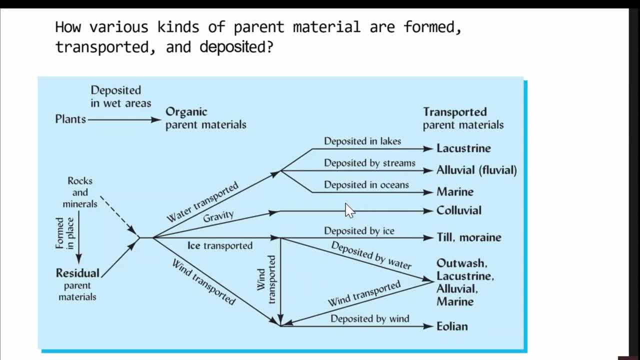 from the ice formations. but if it's deposited by water, it becomes a deposit by water and then it's coming back to the features that you see up here. and then you have winds transport. yeah, wind transport is very easy to see in Oman. not that Oman has a lot of soils, they are deposited by wind, but Oman 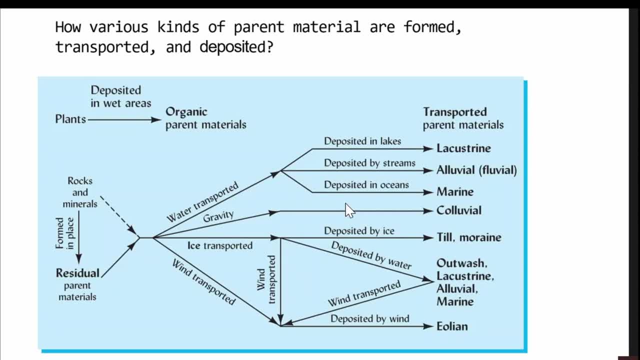 actually is a source of material for other landscapes to form their soils. when you look at the atmosphere here, you see that there is a lot of dust in the air. that dust does not stay here. as the wind goes by it takes it to somewhere else and somewhere else it will deposit and there will form the soils. so we are. 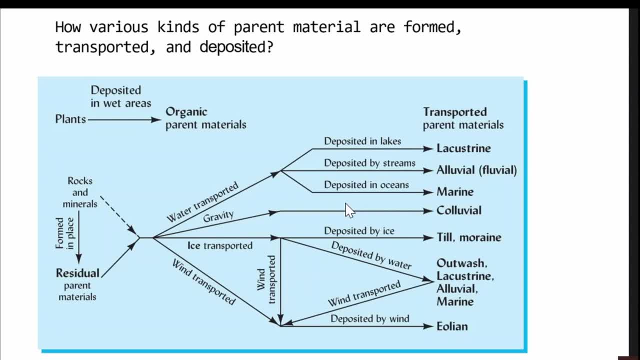 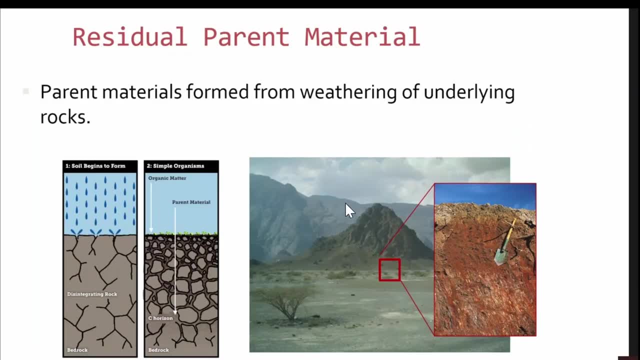 source of parent material for the formation of soils and other regions. let's break down. this is the formation in situ. yeah, whether it's a landscape or not, it's a landscape of underlying rocks. this is rare minute. most of the times you do not see this, just in special occasions. most of the 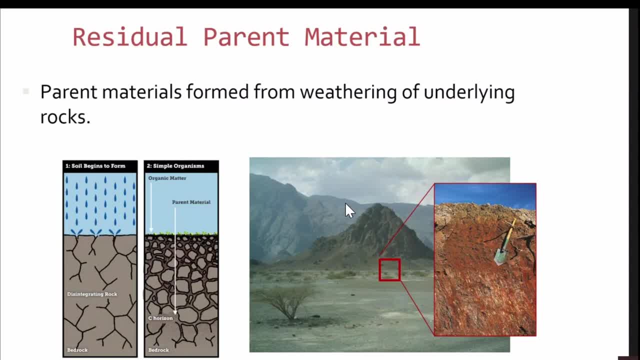 time when you have that, you see the rock already emerging in the soil. shallow soils forming over that rock will have been formed from that rock. but if you have the rest of the landscape here on the bottom, most likely those landscapes are bring by deposits- yeah, fluvial deposits. 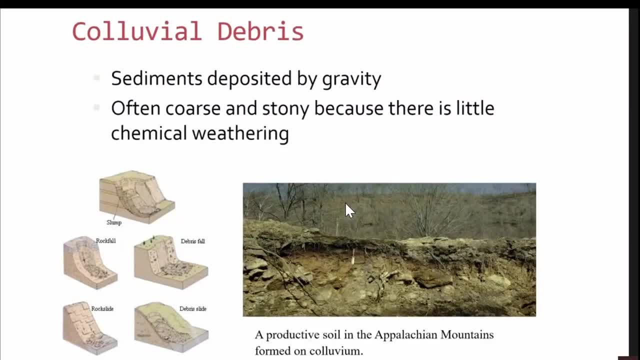 or other types of deposits. so colluvial means that is coming from gravity. yeah, so it's the landslides that I just showed you before, and then you have this clear cut. how do you identify colluvial deposits? first of all, you were close to a very steep slope. then you have a clear break of different aspects. 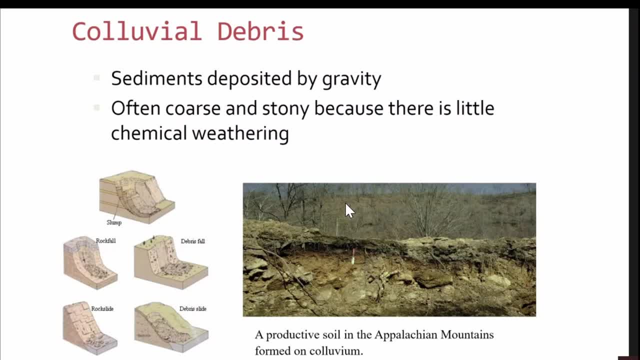 of the parent material. you have a clear break of different aspects of the parent material. you have a clear break of different aspects of the parent material. you have a buried soil below and on top of that you have a deposit where a new soil has formed. so by seeing that clear break between the two types of materials, you 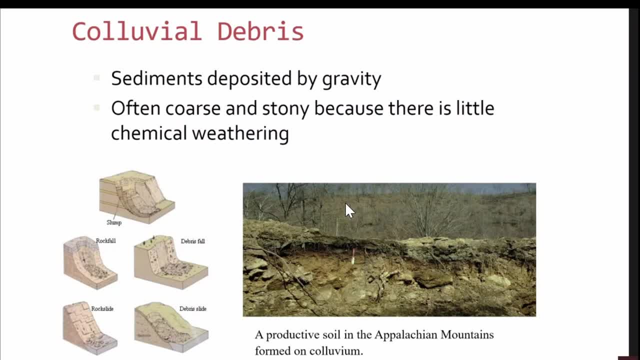 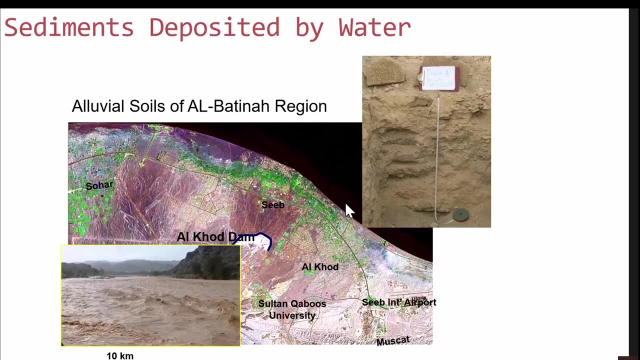 can then assume that if there is the slope, then that is coming from by gravity, by the landslide deposition of the material alluvial deposits. this is the most common one in albatina region. yeah, all the wadis, when you get near the coast they have these alluvial fans. yeah, funds because they 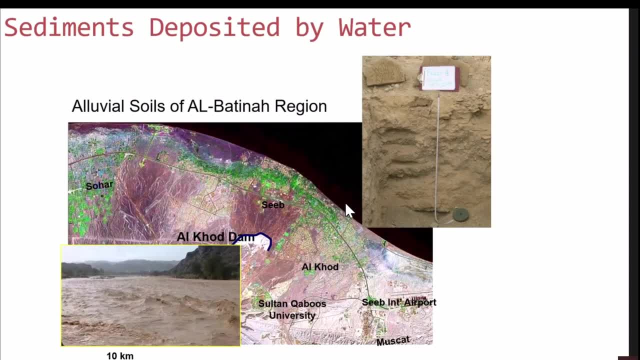 spread out like this. you can easily see here where the one it comes, all the area near the coast where they flood, where the Wadis would flood in the past. that is the area where you deposit. you know they come, they have a rain event, they float that area and then the deposit settles down and then over time you have 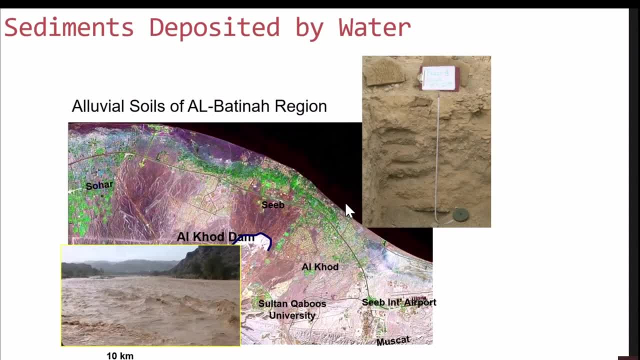 maybe in a decade you have five, six big events, a flood that settles down, and then over time you have- maybe in a decade you have five, six big events- a flooding, and then you take that into a hundred years, a thousand years and you build up a very 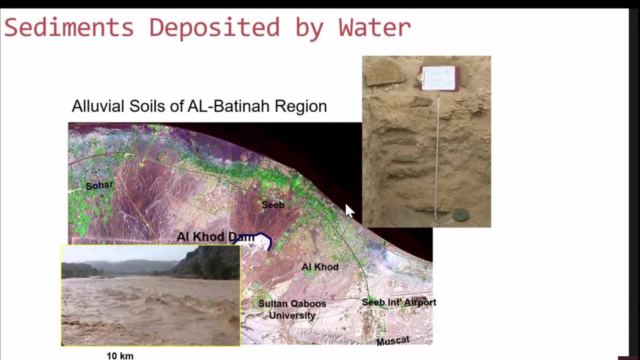 thick layer of deposited alluvial material. so it's very cool that you see that in albatina coast, where you have the wadis, where the slope is a little bit lower, most likely what you have there is alluvial deposits in the soils that are formed. there are usually very young soils. they are not so. 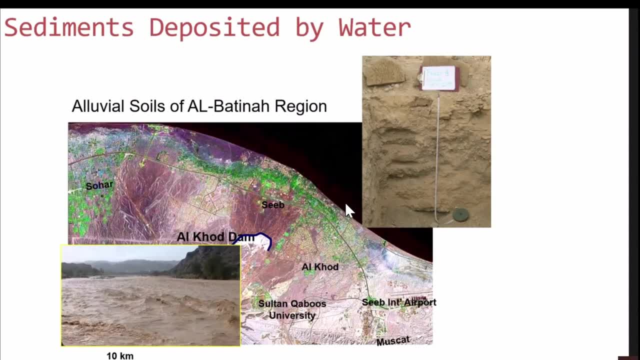 old because the alluvial deposits are constantly being deposited in the place, so there's not enough time for the soil to form. the weathering of the peri material could be high even if the soil is young. why? maybe that material is coming from already other soils that already well developed? 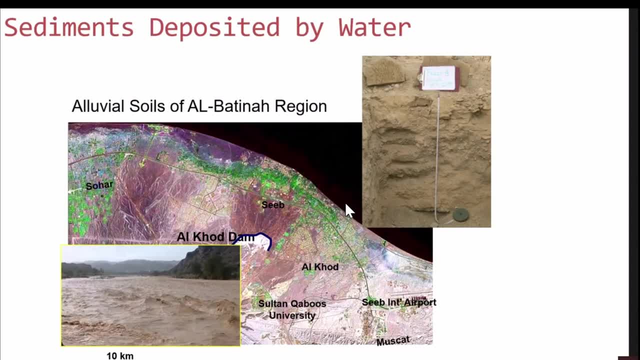 if other soils are well developed and then they're eroded and transported and we deposit, then that material could be already weathered. and what you usually see in alluvial deposits is fine materials, mostly silt. yeah, fine sand silt and a little bit of clay layered. yeah, why layer when you have a flood? what comes down first? you? 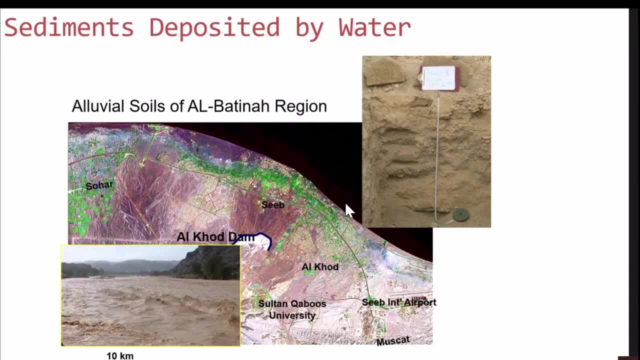 have a water layer. it's a flooded soil. what deposits? first the sand, yeah, then the silt, and then, after a while, the clay flocculates and settles on the top of it. so always in alluvial deposits you have that very thin layered material where you see a gradient of 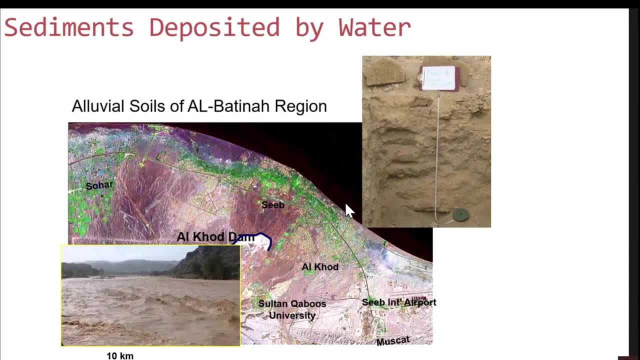 texture. it's coming from craze and becoming finer and then again craze and becoming finer. so this type of formation is a clear indication that those soils are deposited by water, you know, by flugel deposit. so already i don't need to show you images of flooding. we we are very familiar. 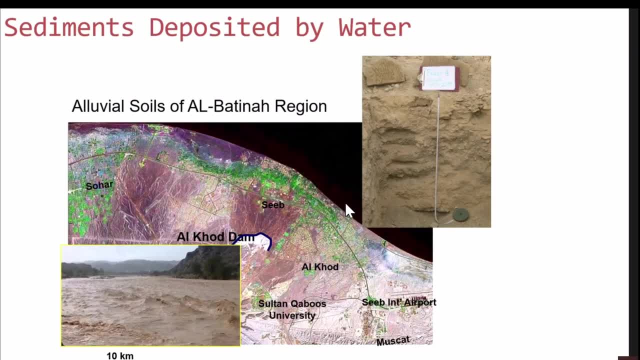 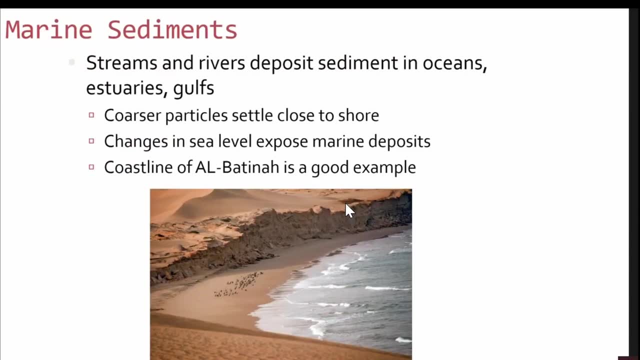 with this. even recently, the shaheen event was very severe here in the batina. marine deposits: yeah, marine deposits are deposited in the ocean. normally, the rivers will bring all these sediments to the coast and then those sediments will flocculate and deposit on the coast, so that's why it's called a high flugel deposit. 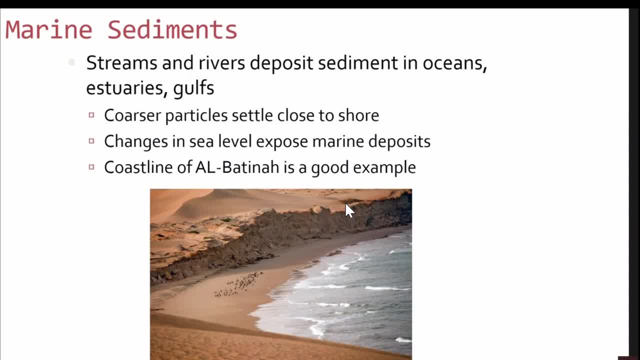 on the ocean bed and then by uplifting, geological uplifting, those marine deposits will come to the surface. in the albatina region you get a lot of that also. you know you have the few, the alluvial deposits, but also a little bit more inland you have marine deposits coming about and they tend 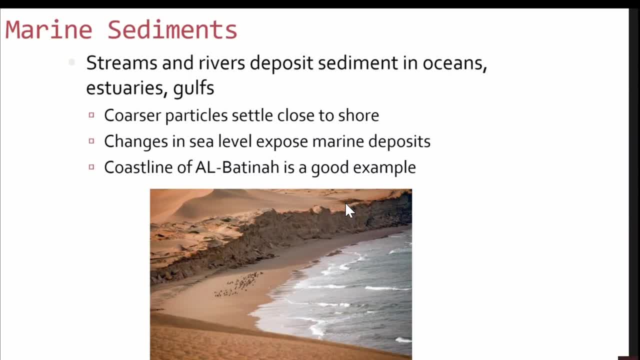 to be more calcareous. yeah, the marine deposit tends to be more calcareous than the alluvial deposits because of the marine organisms and the calcium carbonate precipitation that is happening on the ocean. so the ocean bed will tend to form more calcareous deposits. if you hear, if you near the coast here, albatina, if the 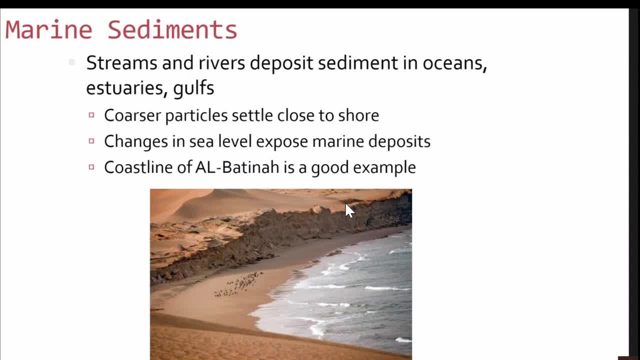 soil is very calcareous. most likely it's either a marine deposit or it's an alluvial deposit that was eroded from a marine deposit. so a limestone was eroded and then it was deposited by the wadis and made the new alluvial deposit. so 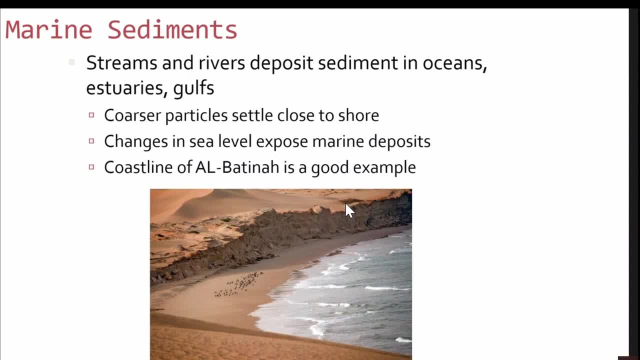 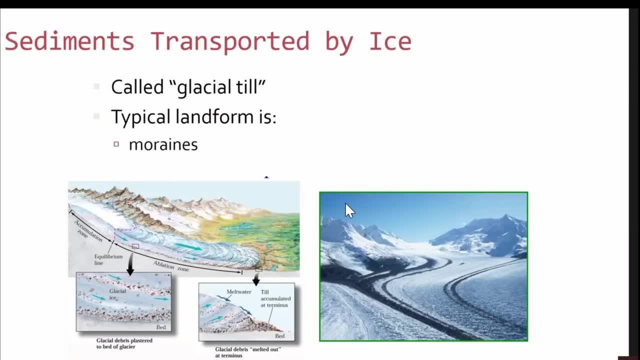 it's already a good tell. if it's the carbonate content of a soil, is already a good tell of the origin of the parent material now transported by ice. that is uh more foreign for uh oman because we don't have glaciers here. but if you travel to mountains- south america, europe, big mountains- you 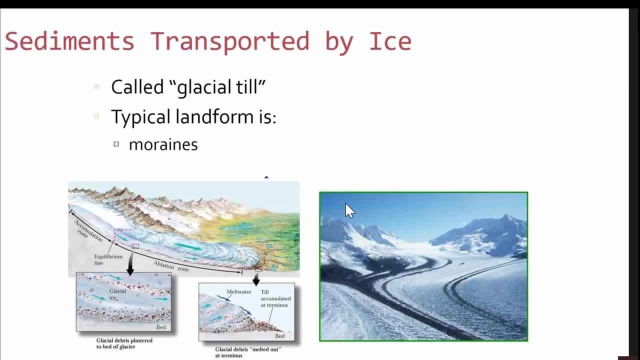 see formations like this, this glacier. they are rivers of ice. yeah, rivers of ice. if you just look at it. i went and visit several glaciers in chile- it looks that nothing's happening, but if you put a camera and take one photograph per day into a time lapse, you will see that the ice is moving down the hill sometimes- let me, the ice is. 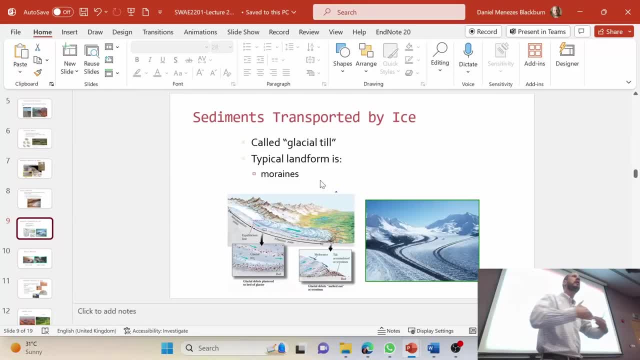 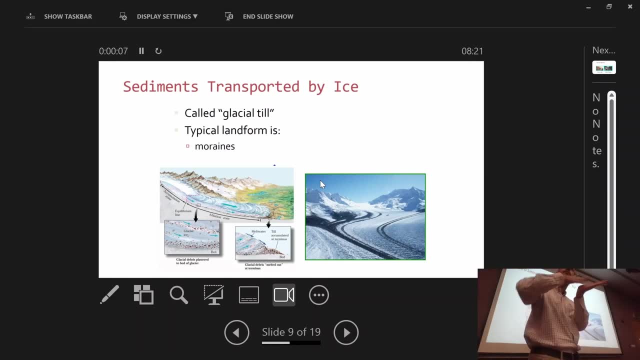 very heavy and below that eyes it's pushing soil. yeah, it's dragging soil with the ice and that makes this ice deposits. not only that, but is fragmenting. you know, the physical weathering by ice is very severe if it's bringing rocks below. rocks are scratching over other rocks and being fragmented, so the physical weather is very severe. 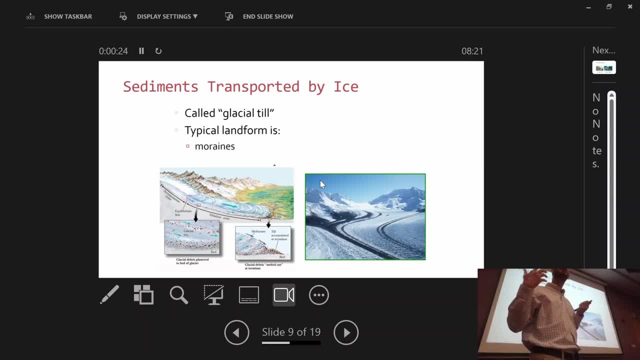 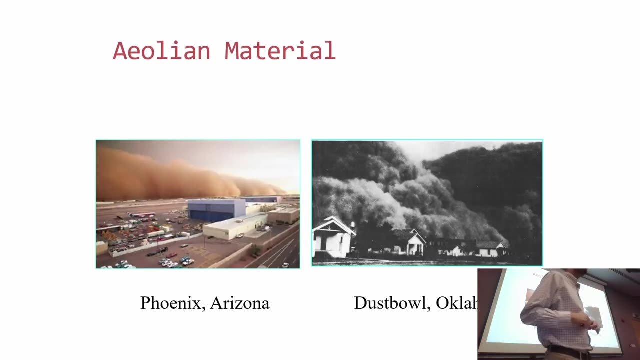 when you have this type of deposits by ice. so not only it's transporting but also fragmenting this material. all right, eolian. eolian deposits are not very common in oman, but in several countries yes, they are. for example, there's long landscapes in china that are eolian silt deposits. 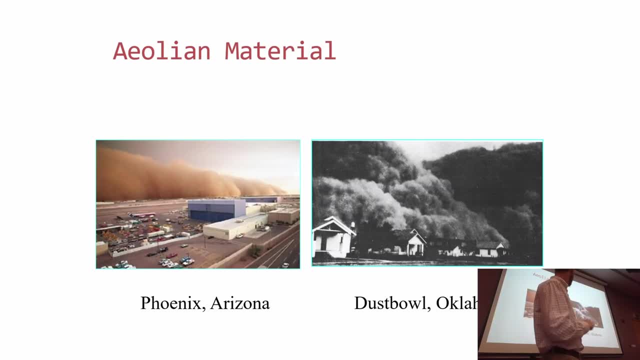 yeah, um, these are some examples of dust storms. dust storms, eolian deposits are not very common in oman, but in several countries. yes, they are, for example, you are familiar with, but then here in oman, most likely you are taking this material and deposited, depositing somewhere else. yeah, 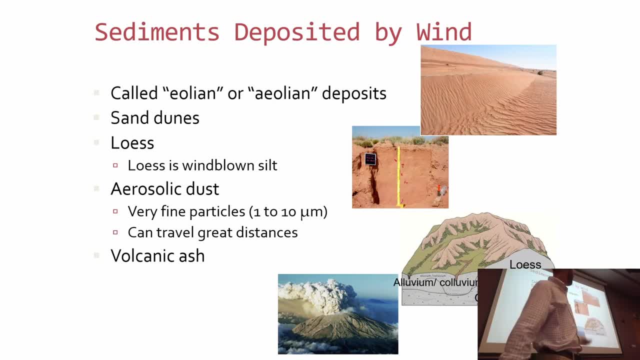 so there are eolian deposits and the main formations that you see, for example the ones in china. they're called lows. yeah, lowest soils are very deep deposits that are coming by wind. most of it is silt volcanic ash. i would even not classify by by by wind, it's just volcanic deposits. yeah, it's a. 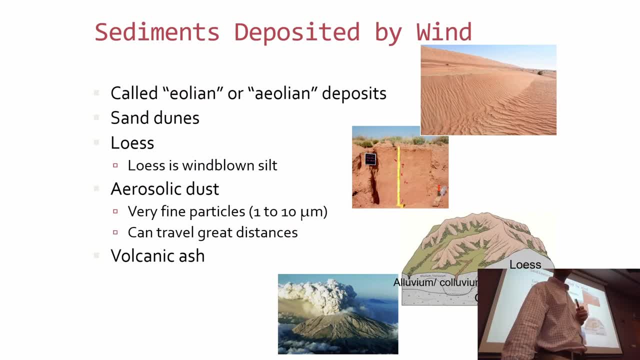 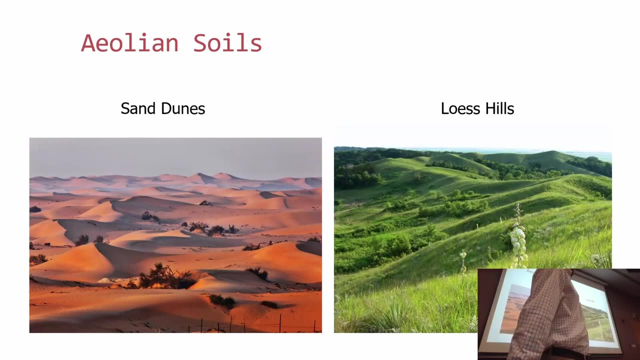 different category altogether: volcanic deposits. but the lowest is the classic example for the eolic deposit. they have very deep soils, very fertile soils, agricultural soils mostly composed of silt that is deposited by wind. sand dunes also can be, you know, if they're mobile sand dunes, they 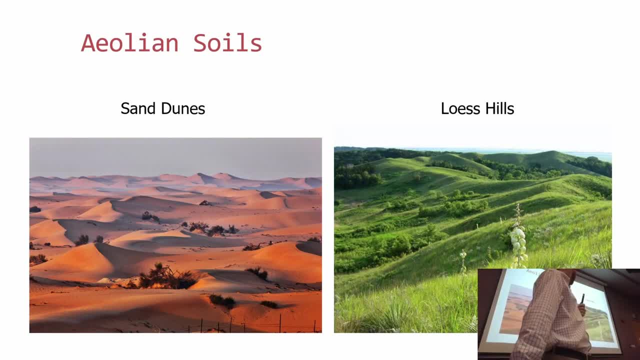 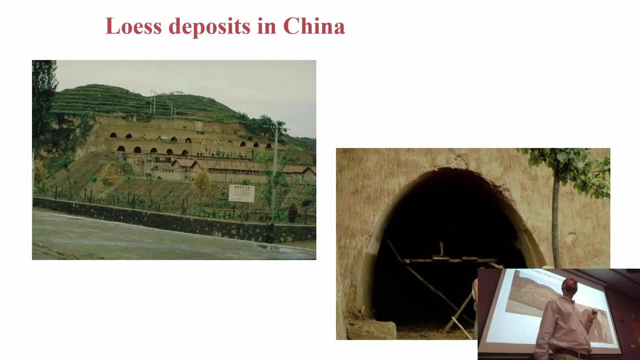 are wind transported and deposited. these are the types of lowest hues, yeah, that you can see, and also these lowest deposits. they they are very stable and you can dig and carve caves on them easily underground. so you have this type of formation of that you can dig and find, you know. 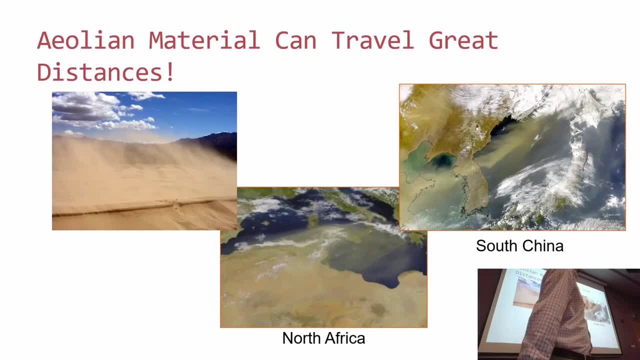 use it for caves most of many times. one of the characteristics of eolian deposits is the parent material. the rocks that they originated from can be very, very far away. for example, some of the dust coming from the sahara can deposit even in south america. and 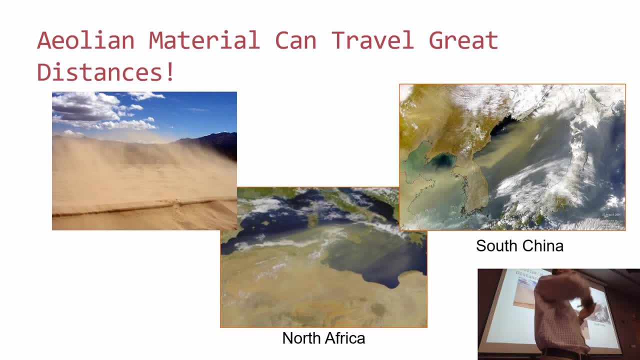 central america. they can travel far away across the globe and deposit somewhere else. the long distance deposits, more than being very important by the the mass of the soil formation, they are very important also for sharing the soil and the soil formation. they are very important also for sharing. 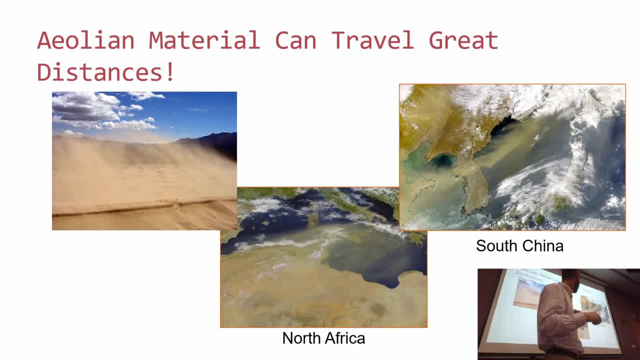 for sharing the nutrients and making that bio geochemical cycle of the nutrients being carried far away. for example, many rocks do not have phosphorus. plants need phosphorus for their nutrition, but calcareous soils from marine deposits they have high phosphorus if they are eroded by wind and they spread throughout the globe. now they're sharing. 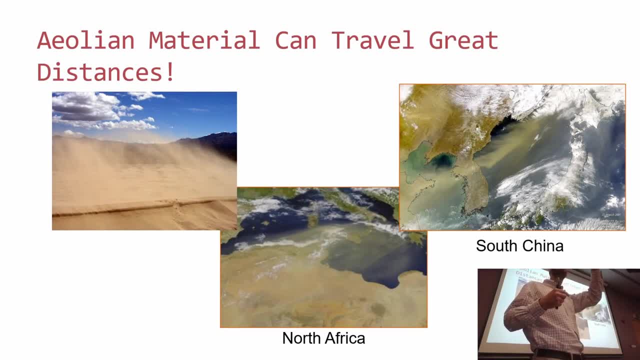 that nutrient. with other soils they have the small mass of deposits. but that small mass of deposits and caused foroshi to intervention, could mean a lot for the nutrition of the vegetation in which they are arriving. okay, But many times they can go around the globe. 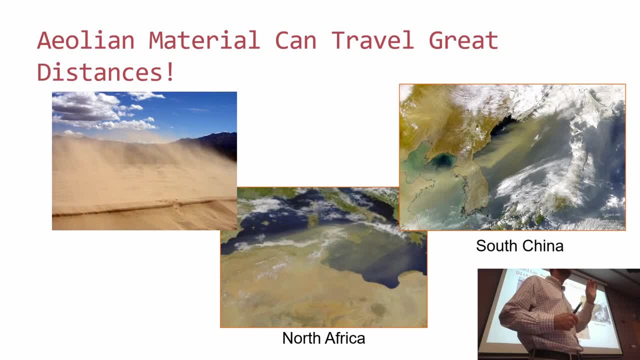 more than once before they are settled, depending on how fine they are. If they are very fine, think about when you have these volcanic activities. the ash goes around the globe dispersing and they are taking a long time for settling. Same things go for this type of storms. 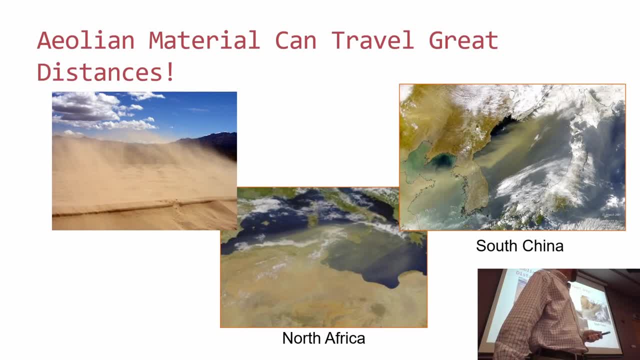 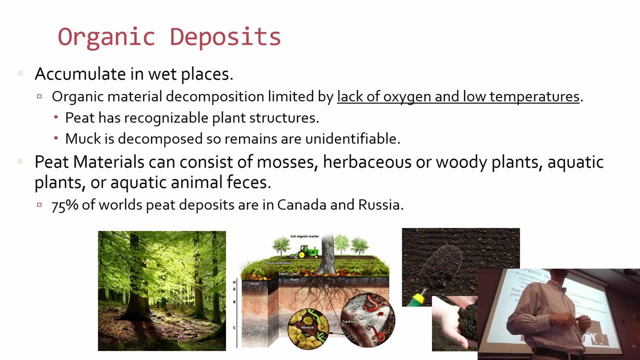 The finer the material, the longer they travel. Organic deposits: yeah, organic deposits are usually formed when you have anaerobic conditions, So you've had dying lakes. swamps then is where you find and form these organic deposits. Also, these organic deposits are more typical. 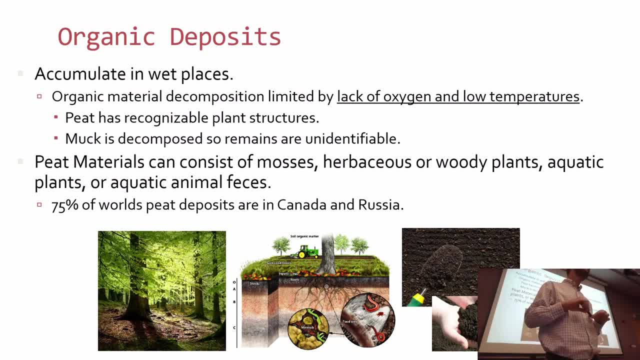 from cold climates, subtropical climates. In Oman, you do not see a lot of organic deposits, first because it's trying, Second because it's hot. Yeah. So cold climates, very wet climates, Flat landscapes where you have constantly wet situations. 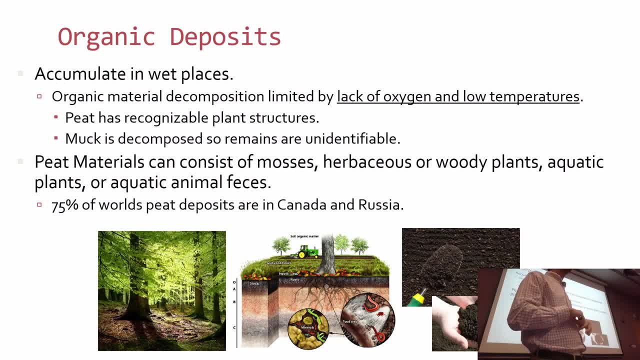 there is where you get these organic deposits forming And over time you get the thickness of, you know, 20 meters, 50 meters of formation of these organic materials. Now, when you buy the peat moss that you buy on the nurseries, 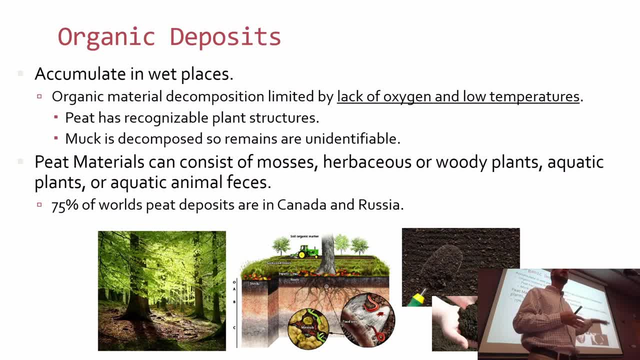 you're. actually, this is mine material, this is soil, organic deposit that was formed over thousands of years, and then they just go there, dig them out, sieve it and sell it for you, for your plants. yeah, some of the characteristics of this organic deposit is they're usually very acidic. yeah, 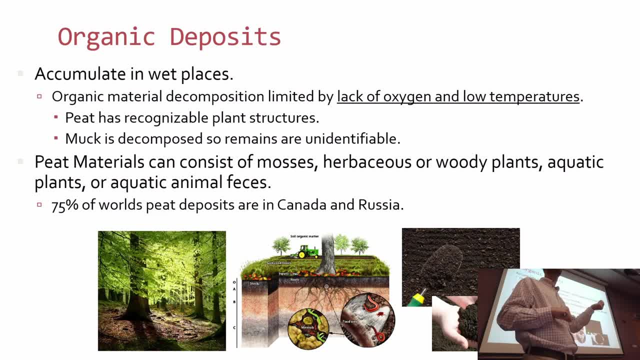 they're acidic. so when you buy peat moss, that peat moss probably the ph is around four, four point, five, five. they're not. they're not very high ph's because the decomposition of organic matter releases protons. so that is a natural consequence that you acidify that material. 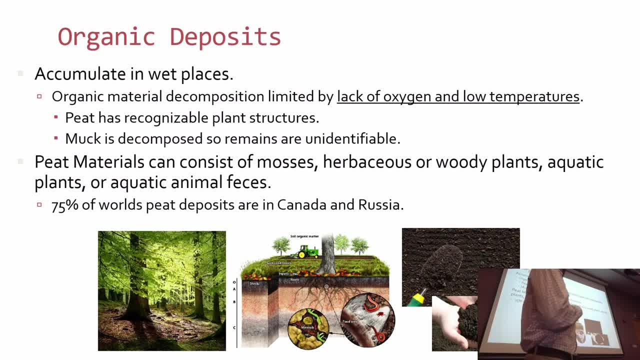 all right, the is a textbook definition. if it's really well decomposed and you cannot identify the plant material in it, you call it muck. yeah, if you can't identify the plant material in it, you call it muck. yeah, if you can't identify the. 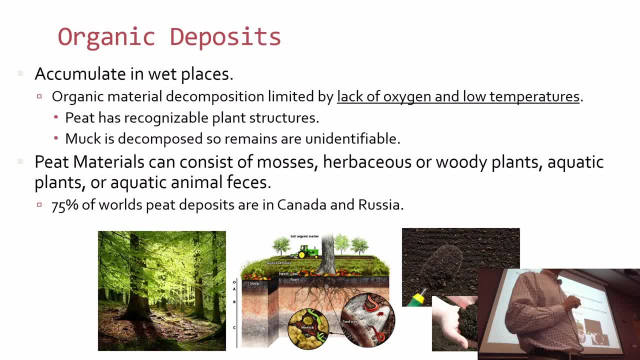 Plancy Mock in it. you call it a different material and you can't identify the fresh, can identify the original material. you call it peat. yeah, now, in general, even the ones that you cannot identify, many are just calling peat all the time, not calling muck. in general, the type of plants that form these type of materials. 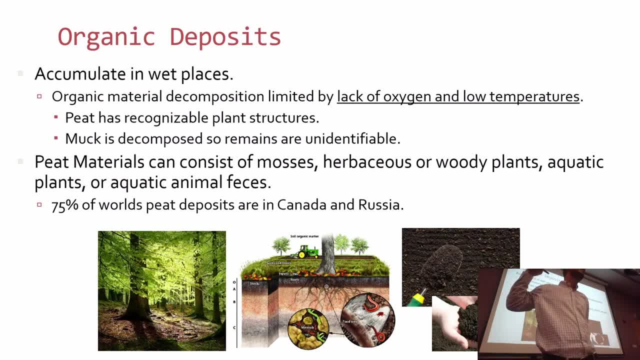 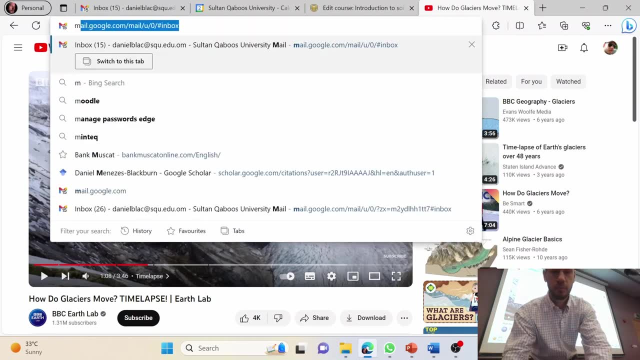 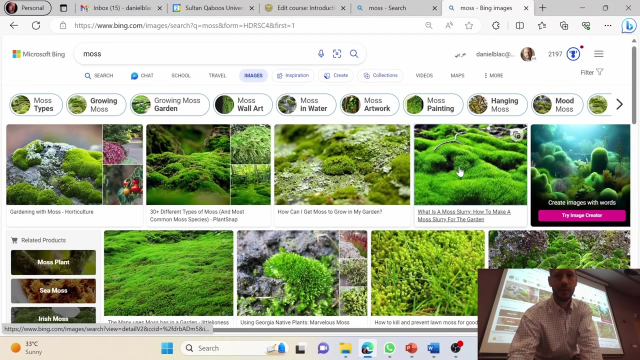 most of the time they are in subtropical climates. it's moss material. yeah, have you heard about moss? you know what moss is? what is a moss? let me go back to Google images. so this is a bri of the type of plants. there's no non flowering. 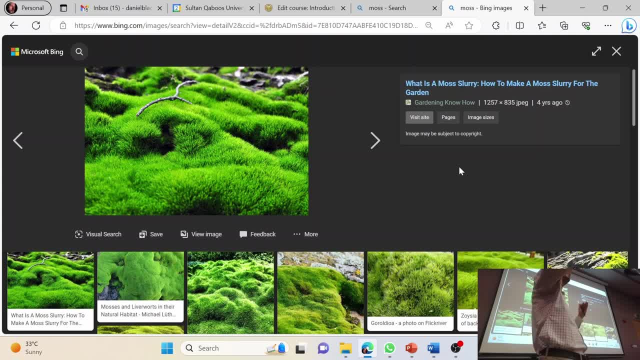 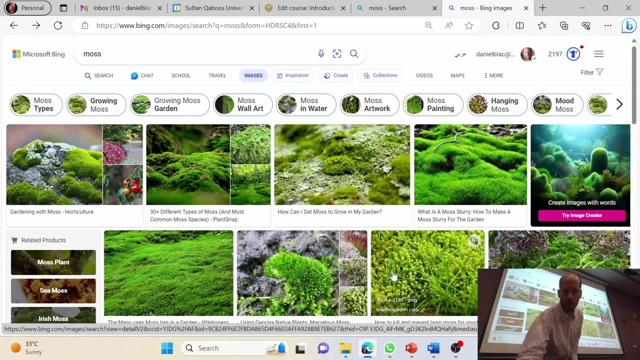 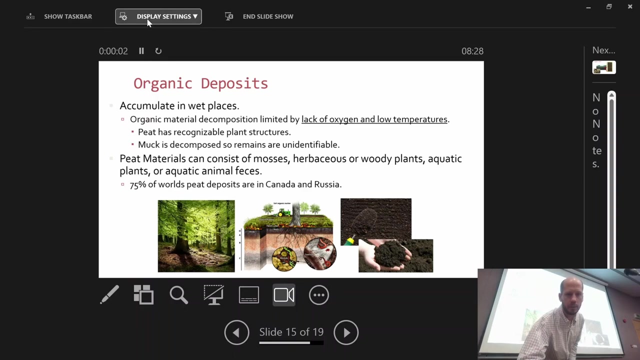 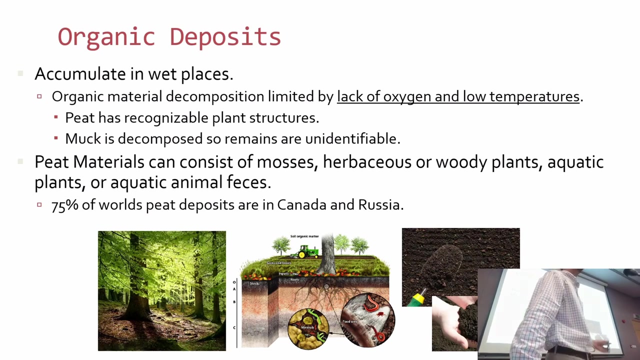 plants that they just grow a layer, then they grow a layer on top of it and they grow another layer on top of it and therefore the layers are stained below. they are being very resistant to the composition because of anaerobic conditions. okay, let's go back. so these are typical from cold climates. in wet 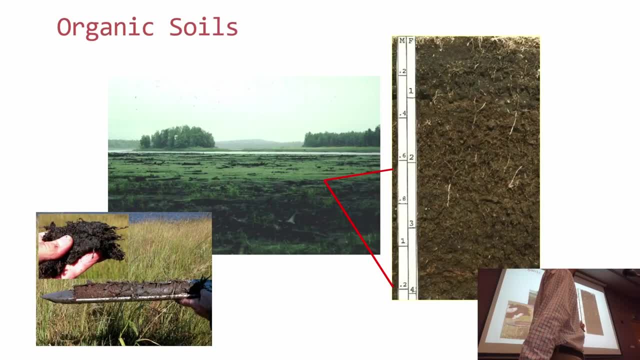 climates: cold climates and wet climates. this is the type of landscape, yeah, flat, cold, wet and, as you form the accumulation of organic matter, some of these soils are frozen by that, by the way you call permafrost. yeah, so there's a lot of organic matter trapped in frozen soils and as you, as you thaw them up, they start. 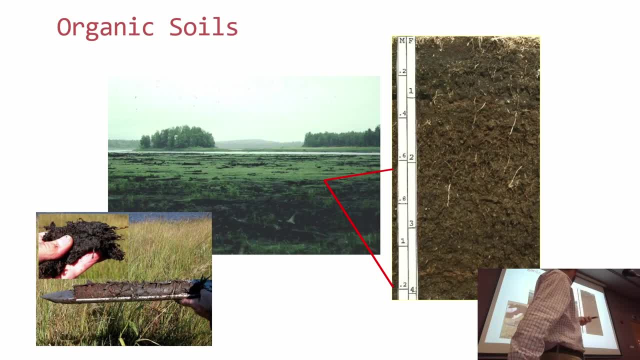 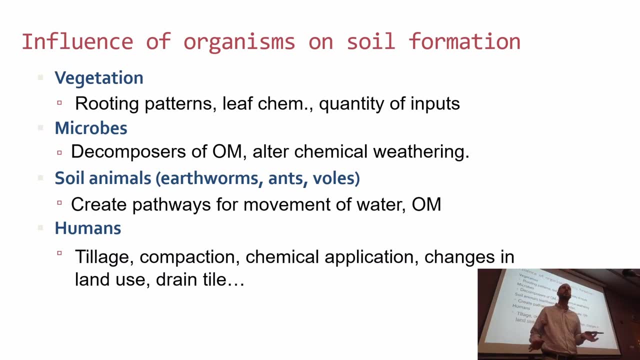 decomposing again and emitting that carbon back to the atmosphere. so that was it for parent materials. okay, we have all the rocks, the weathering of rocks, the transport, deposition of rocks, and there is where you get the formation of soils. now there are other things, you remember. there are other things that are. 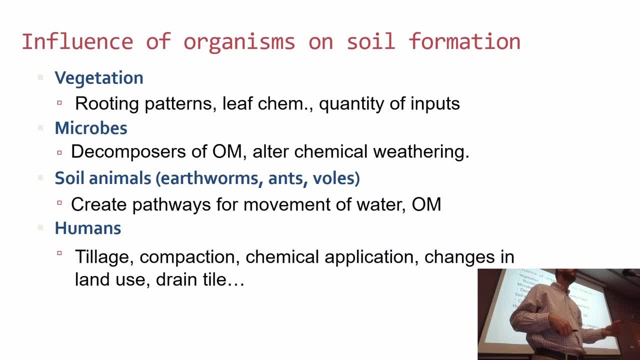 also acting on the parent materials to form the soils. remember the seaport? yeah, climate, parent material organisms. yeah, climate relief in time. yeah, climate relief in time. so let's talk about organisms. how do you say organisms affect the formation of soils? how do you think organisms are acting on the material to develop that we already talked about? 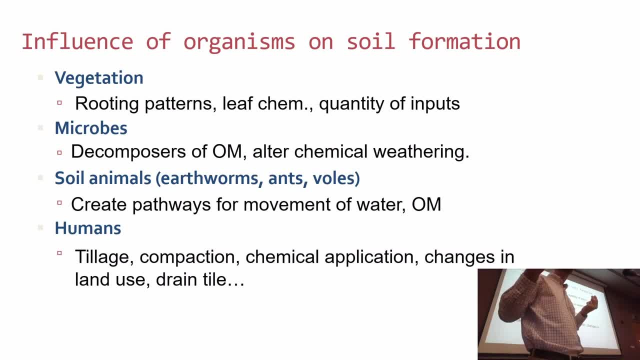 kamu can, can use, can produce materials, produce organic materials. okay, they are depositing carbon on that and, sorry, renewable the soil. renew, how produce some materials to have the soil- maybe it's new, okay, yeah, so they're creating more organic materials, depositing new organic materials in the soil, but 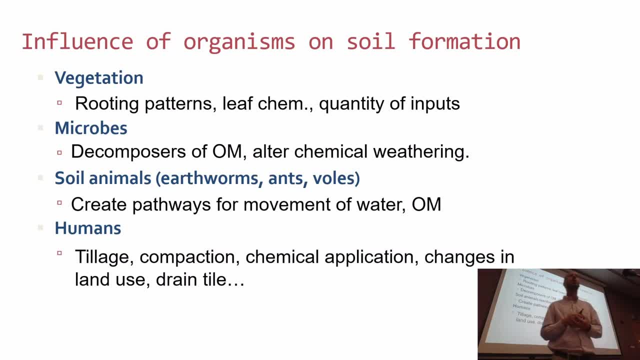 most of the of the situations. every time you have microbes, every time you have plants, they are actively conditioning the chemistry of the soil. they're releasing enzymes, they're releasing acids, they're changing the ph. why are they doing that? for once, they want the minerals, so they are. 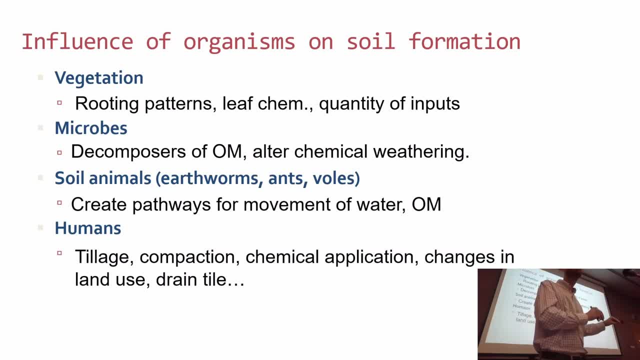 actively acting on the chemical weathering of the soils, so biological weathering is, most of the time, chemical weathering. they are actively acting on the minerals so they can take the nutrients out of the minerals they are interested on growing. yeah, selfish interest in growing the minerals. 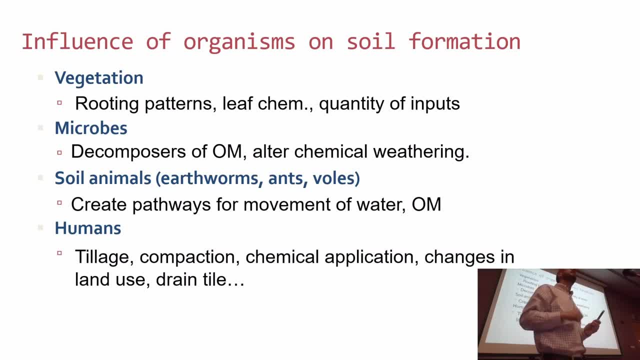 contain the elements they need for growth. they go there and decompose those minerals for their own selfish growth. as they do that, they are accelerating the formation of soils. yeah, their organisms are accelerating the formation of soils actively by changing the chemistry. they release enzymes, they raise organic. 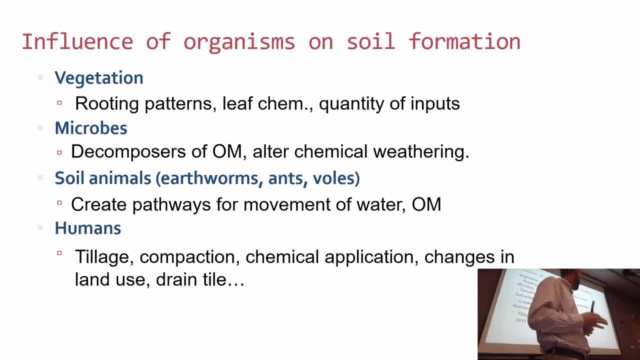 acids, they change the ph and that's mostly it. yeah, so the types of organisms that you will have here working on soil formation is vegetation microbes, yeah, animals and humans. yeah, this is a special topic here. we could make a lecture on that, about entropic soils, how humans are forming soils- yeah, so what we described before, 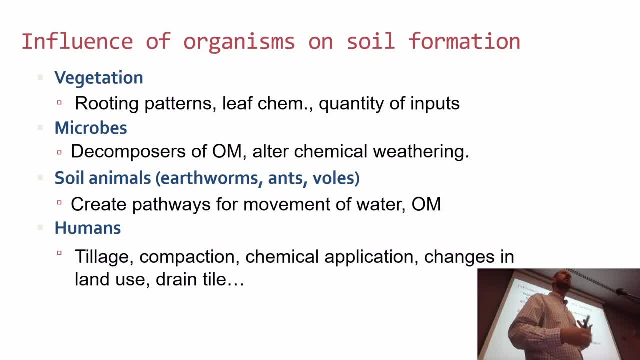 vegetation and microbes. they are changing the chemistry in the soil. yeah, animals- i will put this aside, so focus on the class. so, animals, they are moving and borrowing and changing and mixing the soil. yeah, earthworms, for example. uh, you know borrowing animals? yeah, like ants, walls, they are creating channels and 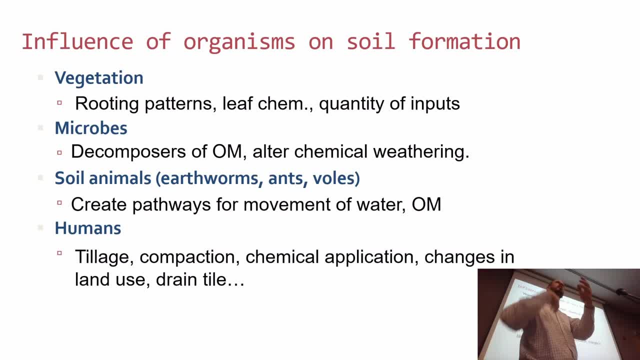 mixing the soil. so not only is the chemistry, but also that effect of mixing humans. on the other hand, you have a whole lot of different other effects. you know, for example, we can actively create a soil just by making a terrasse, for example. there are a whole, a bunch of different. 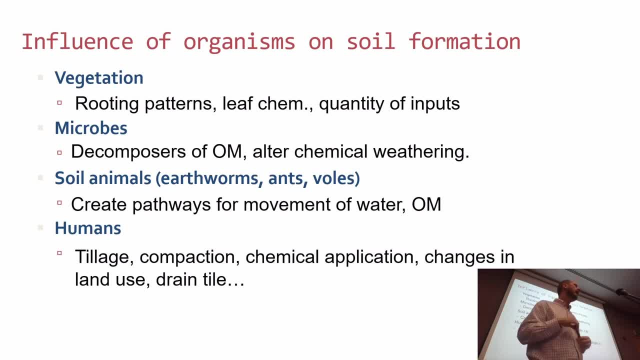 types of human-made soils. we actively seek to form soils throughout our history because we are interested in agriculture. it's not only that we are plowing the soils and mixing them, but sometimes we are making these soils from scratch. there's nothing there and then you start, you know, adding some material slowly, because 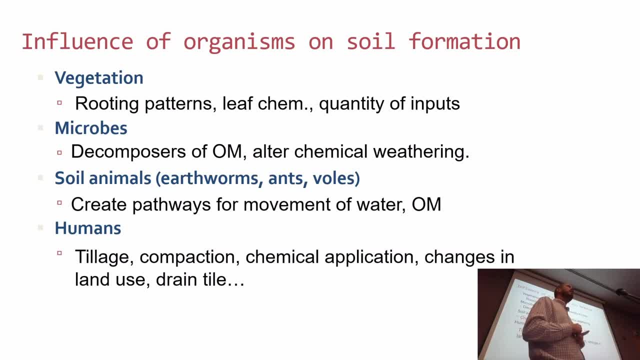 you're interested in growing stuff there. one of the examples we have, for example, is in the amazon forest. indians on the past thousands of years ago they were actively adding charcoal to the soil to increase the soil fertility. they're making charcoal and they're adding charcoal for the soil and the soils. 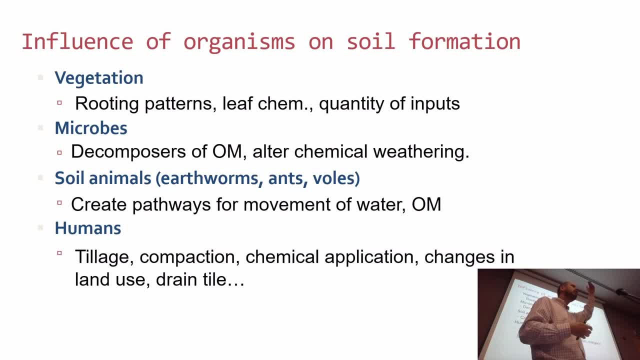 become more fertile because of that. now, when you dig and describe the pedon, you have a clear cut where this, the entropic soil made by the indians, and the other soils were nearby, which is the same origin of parent material but did not have the entropic influence. 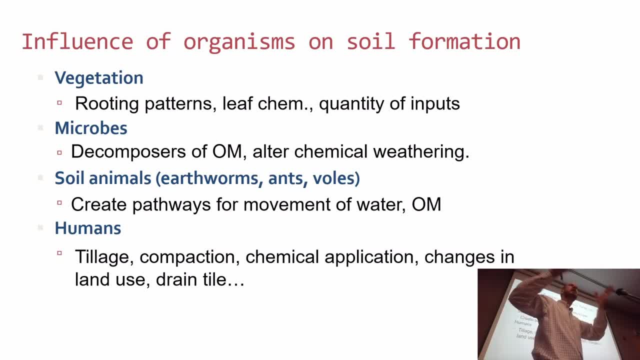 only the vegetation is one soil. vegetation and humans is a different soil. okay, so humans can change that. if you put that over time and you can identify in some regions over thousands of years, you will get that where the humans are acting upon, the soil is a completely different soil. 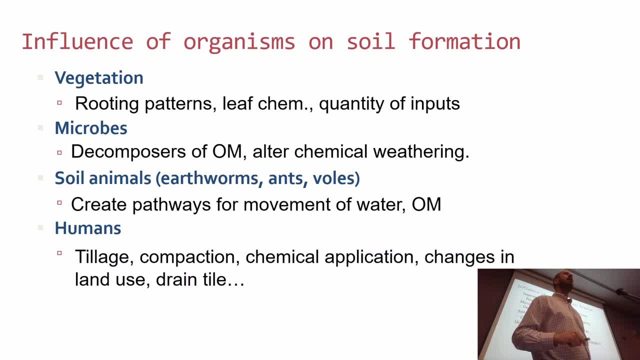 where you do not have it. so this is called- we put here together with organisms, but could be a different category completely- the entropic formations of soils. yeah, entropic soils. there are many different ways in in which humans can affect, but every time we are doing agriculture or trying to use the soil for agriculture, this is most of the time where we 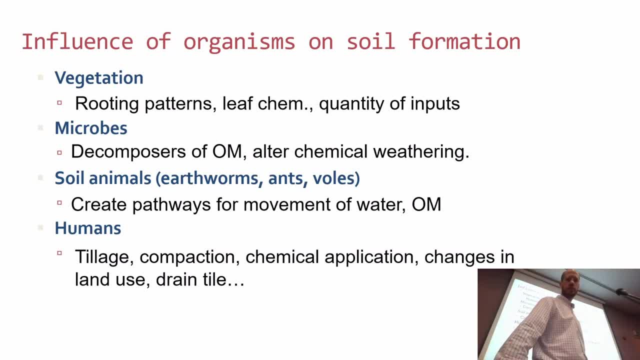 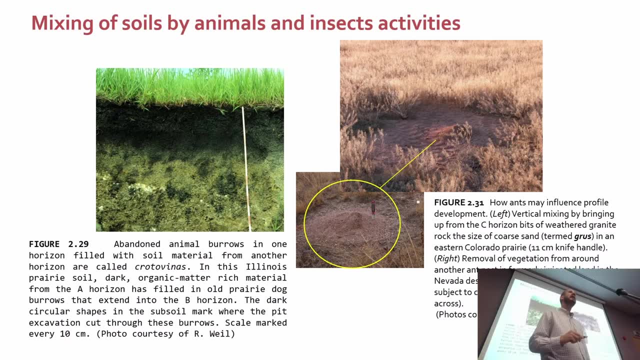 create the soils. so here are examples where you have mixing of the soil by organisms. if you have a soil where there is no organisms that are mixing, probably the top soil would be only 15- 20 centimeters where the roots are mostly concentrated. but because you have earthworms or other organisms that are mixed in the soil, 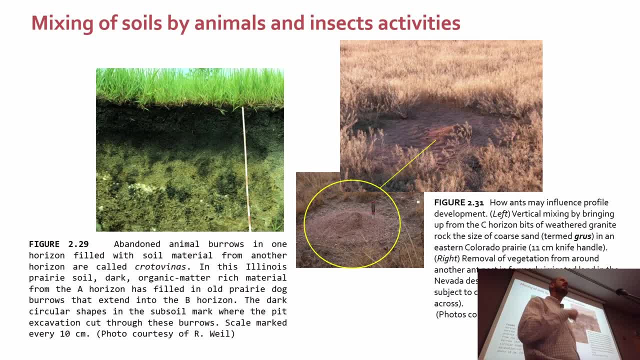 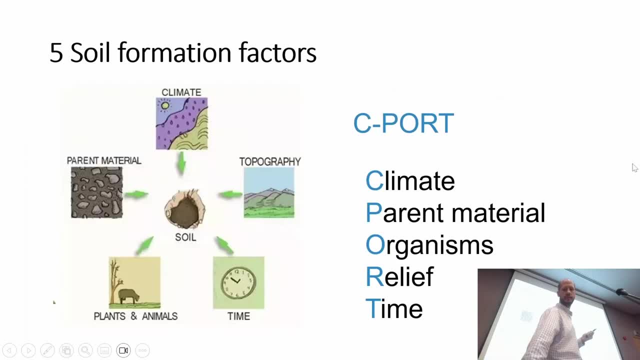 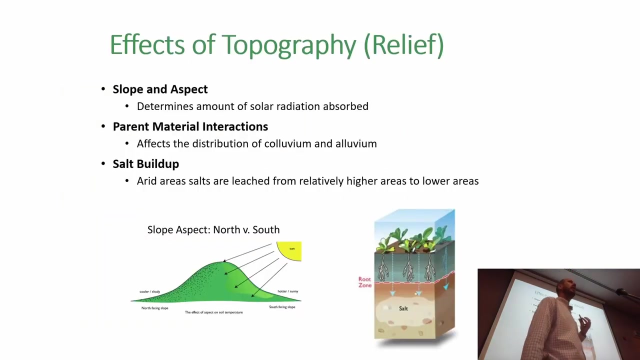 you get a much thicker a horizon because of the the action of these animals and insects. next will be climate relief and time. okay, climate relief and time. in order. here it's relief, not climate. yeah, what is the effect of relief? how do you think the relief? you understand relief, by the way. 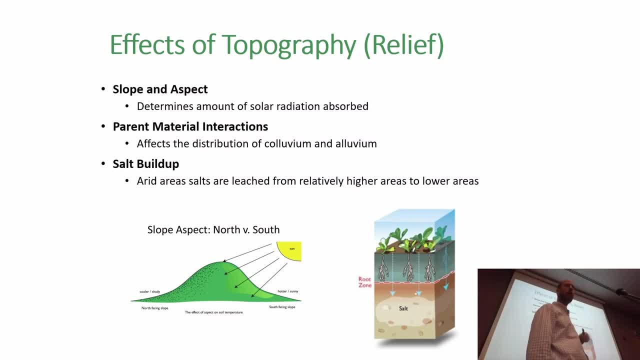 there's two components of relief. yeah, you have the slope and you have the aspect. yeah, slope it means high slope, very inclined low slope, low low inclination aspect is the orientation. the closer you are, for the the equators, the aspect is less important. it means that from both sides of a hill you will get the. 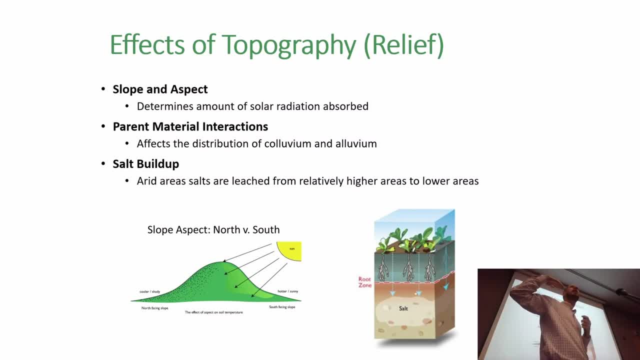 same exposure of sunlight. uh uh, condensation- yeah, you get similar conditions. but if you are further away in the north, you will get the same exposure of sunlight. it becomes more important that sometimes if you have a south facing side of the hill, it's completely different from the north facing. you will get completely different exposition for. 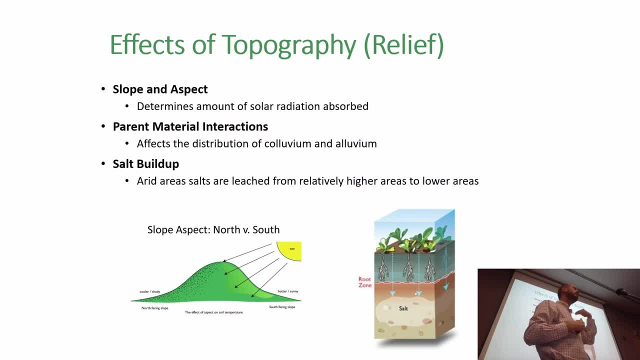 the elements. you know the temperature will be different, the amount of shade and sunlight will be different in one side than in the other side. but as you get closer to the equator, you need to find the special conditions now. even in oman, you will see that if you go, for example, the mountains. 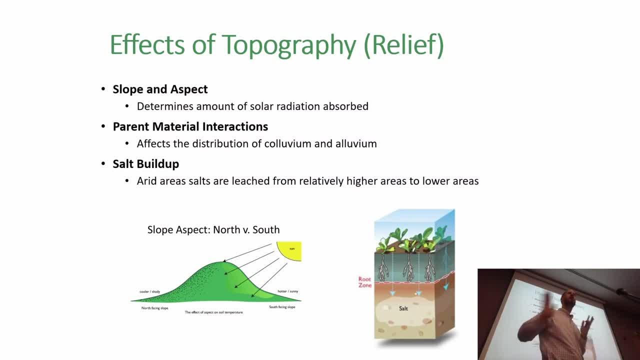 here, like you have jabalachdar and jabalchams and so on, all the mountain, the hills. the side that is facing the coast will have a different exposure for for the elements, as you have on the other side. okay, so relief and climate are tightly related together. in one side you have more condensation. 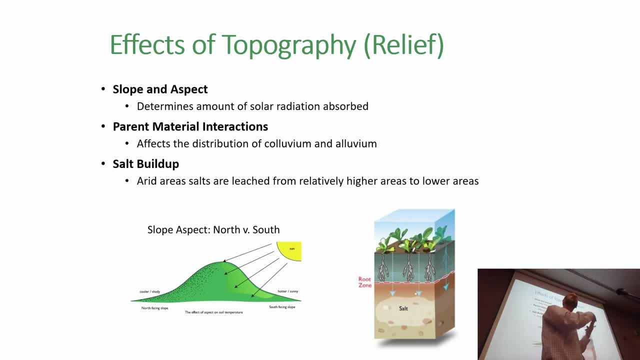 because you have the moisture coming from the ocean and you have condensation. the other side would be drier. yeah, so all of this is a different kind of exposure, for the other side of the coast is affecting a lot how the soils are being formed, because there is a relationship between the 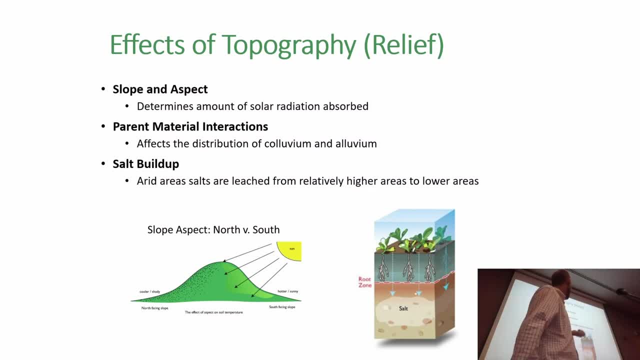 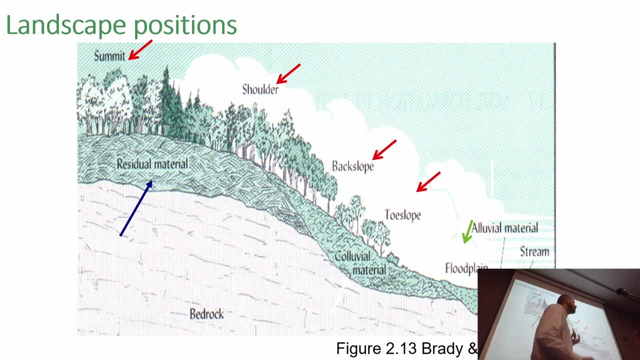 aspect in the slope with the um, what is happening on the soil? the other thing is about erosion. yeah, erosion in the position. so you have this different uh components of uh relief here called in the summit on the top of the hill, shoulder, back slope, two slope and the alluvial valley on the bottom, or the flood plain, flood plain or alluvial valley. 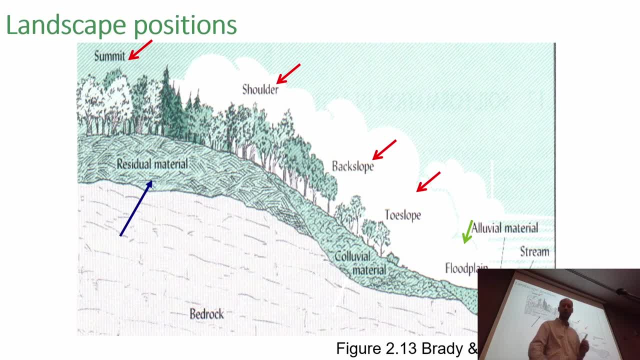 so what do you expect to see? the type of soils happening on these types of landscape on the top and the summit? yeah, on the summit here, probably you will find that the parent material is the rock. the rock, the, it's in situ soil formation, because eroding this material is not a place where you have a likely to have strong deposits. yeah, so if 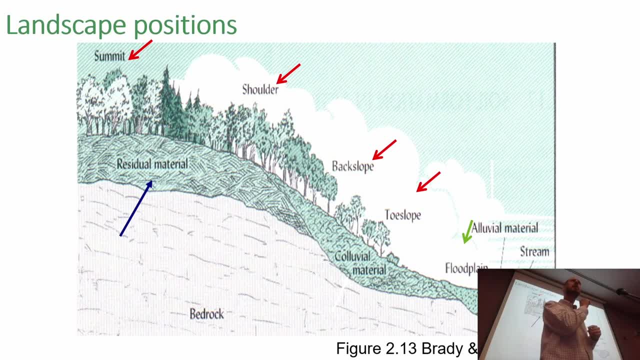 you have underlying bedrock, most likely on the summit and on the back slope you could have in situ formation of soils. so the soils are being formed from the composition of the rock that originates. now on the on the summit, you probably have less erosion, so deeper soils. 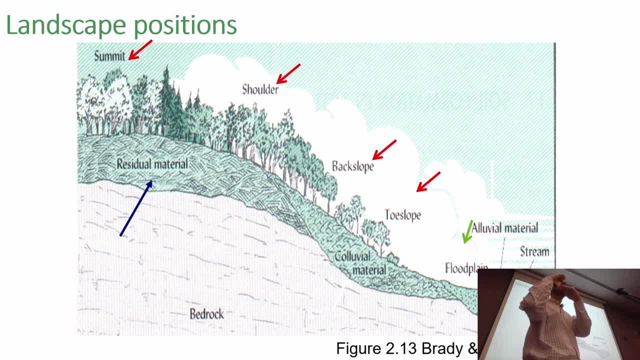 on the shoulder, you will have some erosion in shallower soils. okay. so because of the erosion also you get younger soils on the shoulder. then you get on the summit, the back slope. you can start seeing some colluvial deposits and some soils formed over colluvial deposits, deposited by gravity landslides. 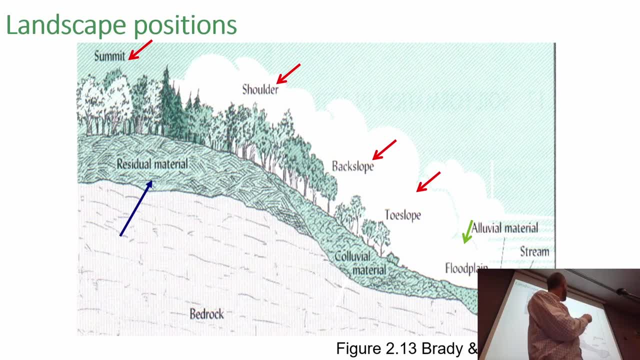 from the past. deposit this material over here and then you have some soil formation over this colluvial deposit. two slides from the past and then you have some soil formation over this colluvial deposit, slope the same thing and alluvial material on the on the bottom, where it's coming from. 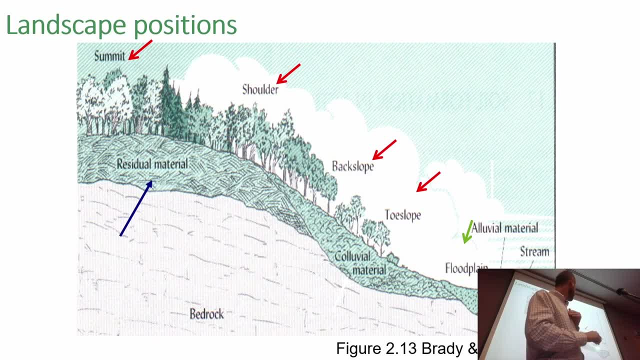 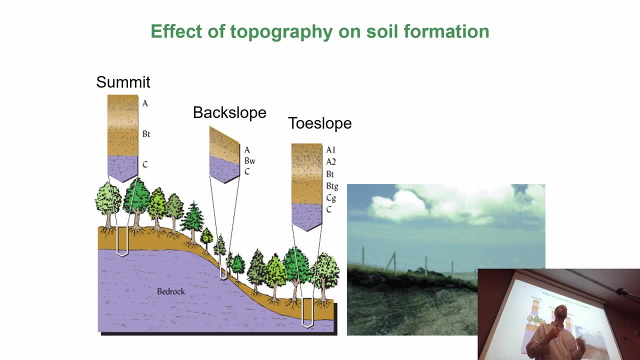 the river, yeah, the floodplain. where the river floods, then you get these depositions over here. so you get that because of that, you have different maturity of the soils and different weathering and different types of horizons that you get in different places of the relief. yeah, when you study, 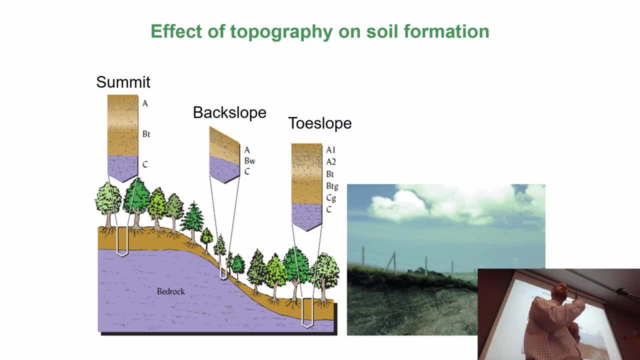 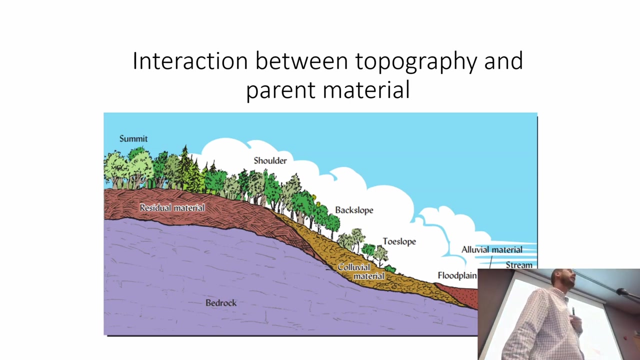 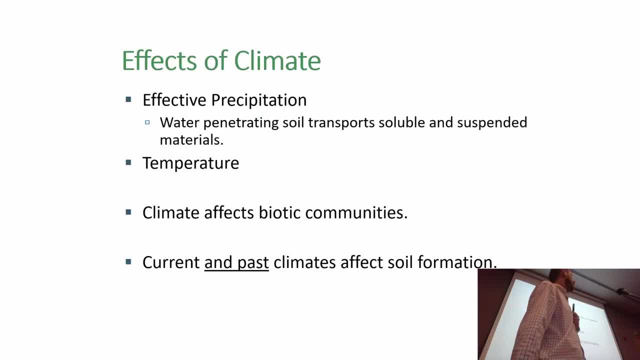 type of parent materials that you have. climate, yeah, climate. you have mainly two different elements that our condition in this. these are tired, yeah, tired, but the different elements from climate that the main ones are temperature and rainfall, precipitation, humidity, and temperature and rainfall, precipitation, humidity and humidity, and 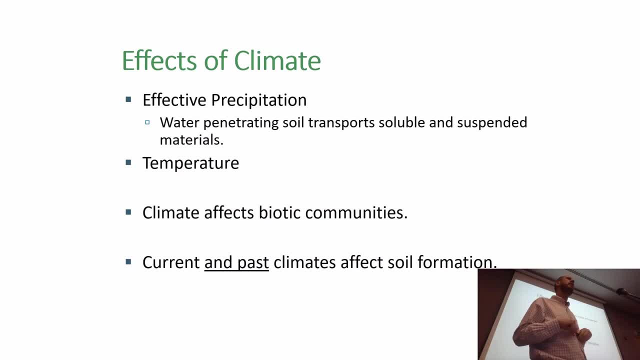 and you have temperature, the temperature. how does it work? for the temperature? let's talk first because of the temperature. chemical reactions, weathering, chemical weathering is proportional to the temperature. every 10 degrees you increase the temperature. every 10 degrees, the rate of the reactions double the rate of decomposition of rocks, the rate of growth or the activity of 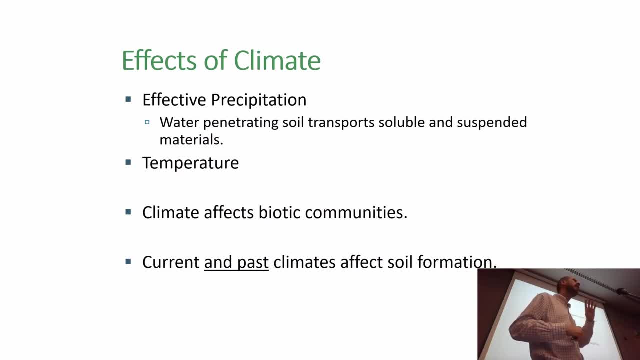 enzymes, any chemical reaction. approximately they double every 10 degrees. so if you have the average temperature of 20 degrees and you have another place where the average tempers, average temperature is 30 degrees, you would expect the rate of soil formation is double because those chemical reactions are being accelerated by temperature and so on, and so 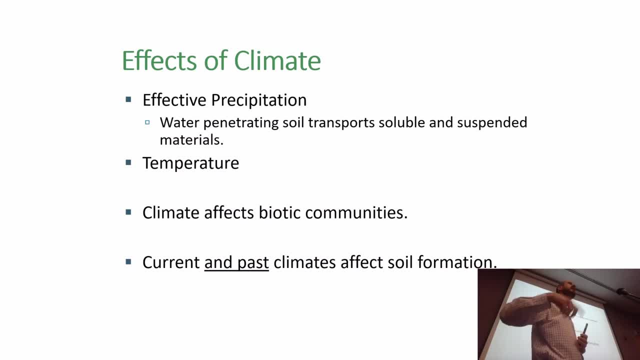 forth if you increase more, if you increase 20 degrees quadruple, you know it's quadruple- double the first 10 degrees and then double again, then the next 10 degrees. so, Oman, being a hot climate, the effect of effect of temperature is an accelerator in soil formation. 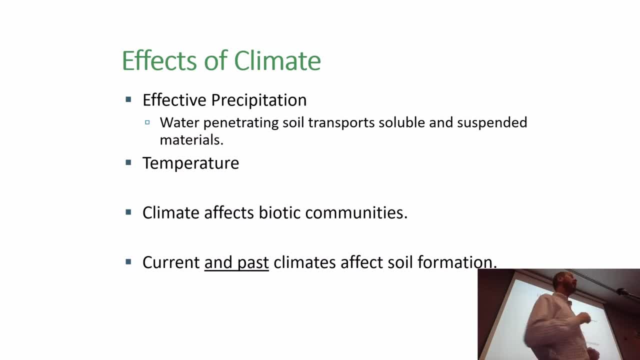 now, precipitation is where Oman will be coming having the problem. how does precipitation affect? it will condition everything else. you have chemical reactions in water. yeah, this though. there is an interface where chemical reactions happen. they're mostly happening in water, all those chemical weathering reactions that we are talking on the last lecture. 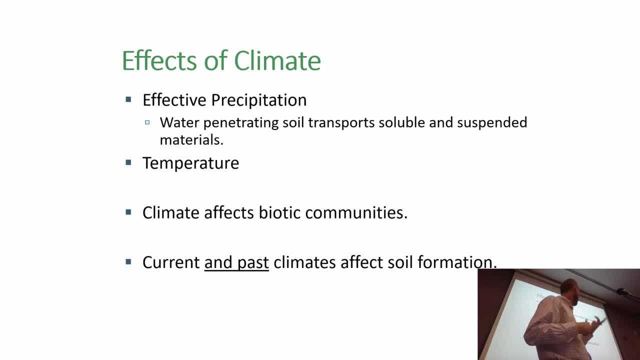 they are occurring in water, hydrolysis, oxidation, reduction reactions in the solution. these are water mediated reactions. so if you do not have moisture, that developed because of the water here and water has an indirect effect on the soil. so, for example, you have an organic soil in a place like Oman, like the atmosphere is very, very, very slow, so in Oman the soils are not well. 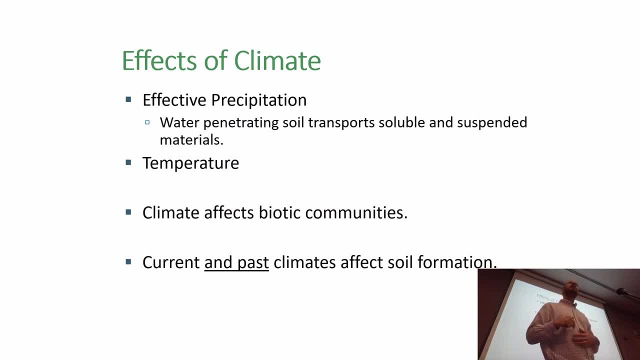 developed most of the time because they are dry. you know there are dry soils. the indirect effect is the climate affects the organisms. if you have more rainfall, you get forests, you get a high occupation of the deposits: organic materials, microbes, plants, animals. if you have a desert, then 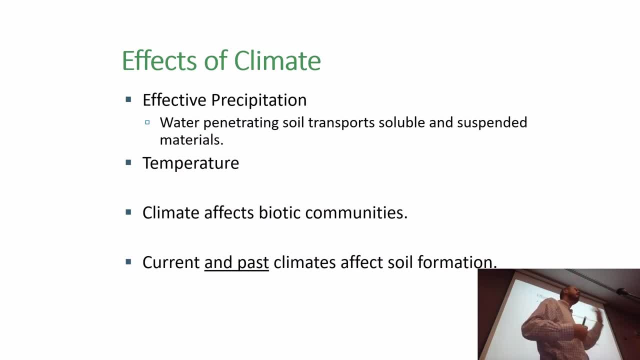 is much lower and therefore these are also not acting on the parent material for the formation of soils. so this is indirect effect. but one of the things that you must consider is that it's not only the current climate. right now, maybe the soil is very dry, but if you go there and you dig the soil and you make a, 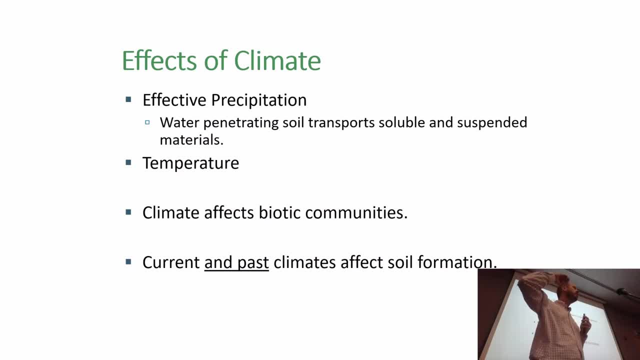 pet on. it looks like a very well-defined soil which has the effect of a lot of rainfall coming through the soil. and why? because maybe that region a thousand years ago was a very wet region. it was a high rainfall. imagine now that you have salala and maybe in a thousand years salala becomes like muscat dry. yeah, but 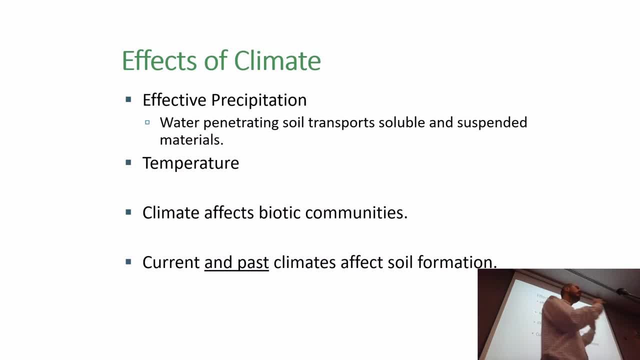 salala has more rainfall in here, but now the soils are being affected by the, the rainfall that you have in salala at the moment. you have more monsoon, but maybe in the future- change of climates and then it becomes a dry region. but if you go in the future and dig the 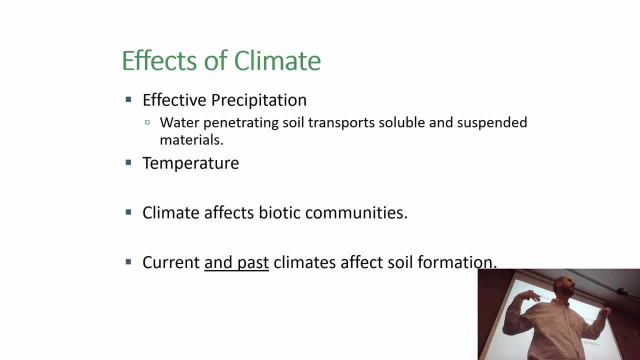 soil. the soils may be reflecting what happened on the past. yeah, so it's not only the current climate, it's a little bit of the detective work you know. you have to go there and imagine what would have been the conditions in the past that led to the formation of those soils so many times the climate. 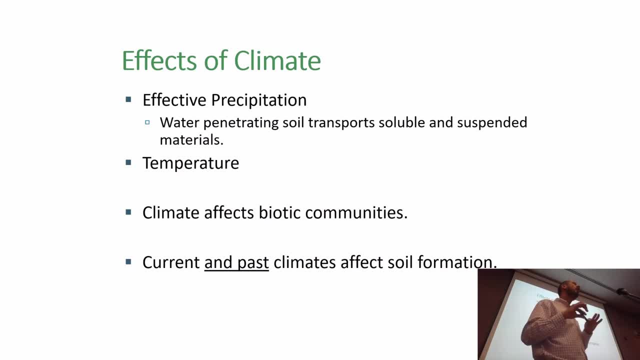 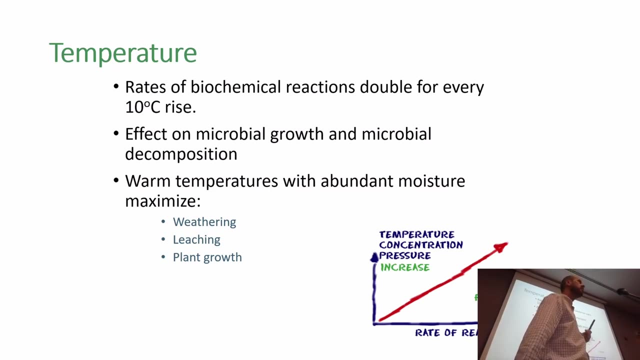 is not the current climate, it's what was in the past. and the older the soil is, the more the best climate is relevant for the soil formation. okay, we talked about temperature. the rate in she doubles every 10 degrees. yeah, conditions, organisms, you know the weathering is faster the more 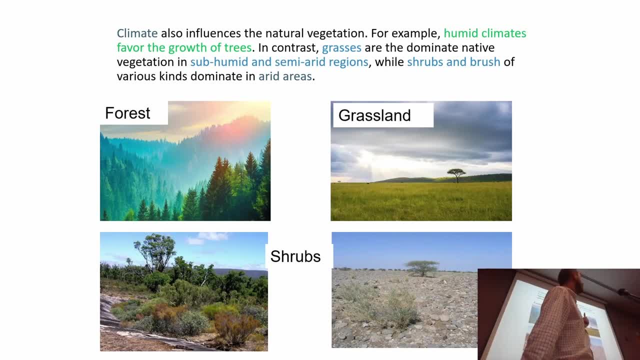 temperature. also, climates are conditioning the presence of different organisms. so these different landscapes that you can see here, they are mostly conditioned. but what type of climate you have on that region? also higher animals will change easily from one type of grassland for forest. so it could be an interaction between climate and the presence of 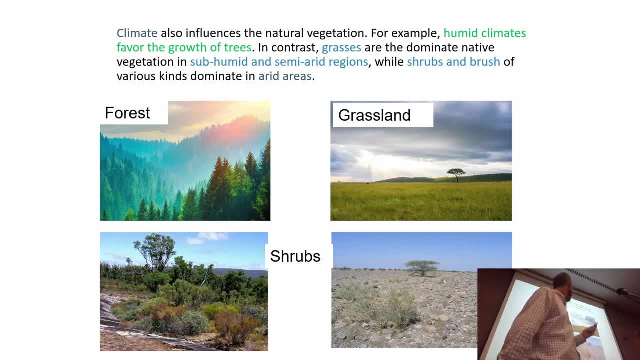 higher animals here also. for example, if you have a lot of grazers, there's a tendency of forming more grasslands and the soils formed under grasslands or different of the soils formed under forests. so let's say, if you have a lot of um, deer and other grazers that are just eating. 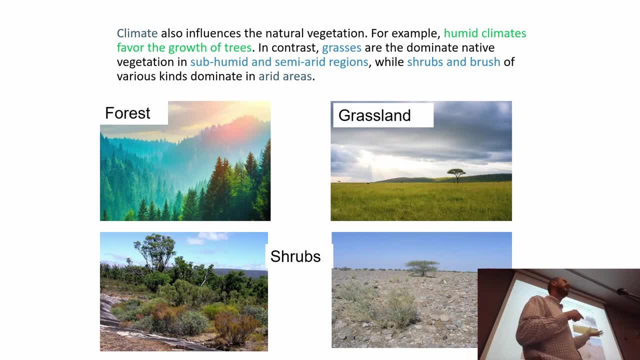 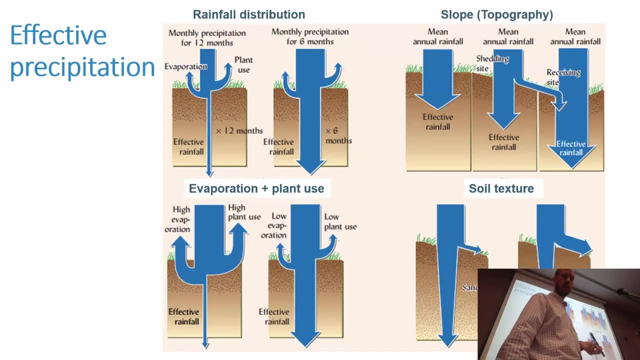 pasture you tend to form more. you know, if those grazers disappear, then you have the more formation of the forest in that same place. precipitation, yeah, you have. the precipitation is conditioning the soil, moisture, the rate of decomposition, but also vertical transport inside the soil. we talked about the b? horizon, the b? 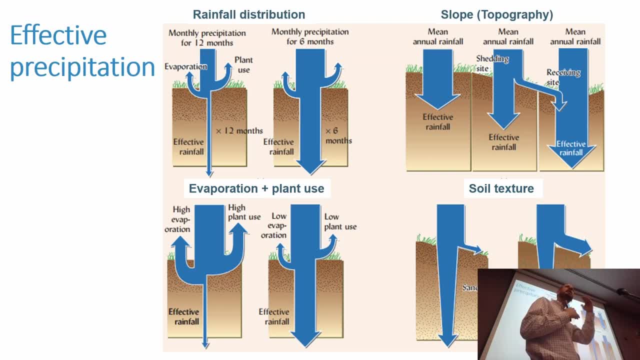 horizon is a deposit horizon and that b horizon only happens if there is water moving in the soil profile downwards. yeah, so it's conditioning the soil formation, not only by having a higher moisture for increasing the rate of decomposition, but also by internal transport and redistribution in the soil. yeah, 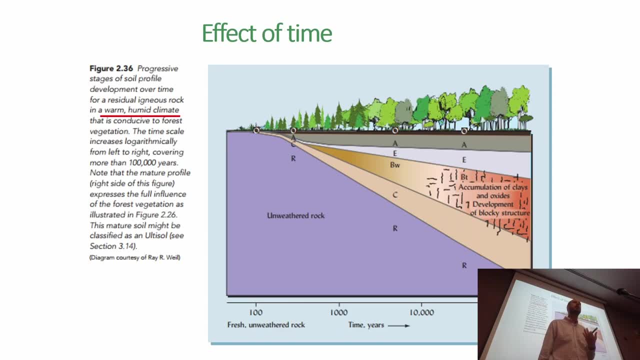 time. time is the ultimate modulator. you have the same parent material. you have the same climate, same organisms, but if it's a recent parent material, it will be a underdeveloped soil. if you give it enough time it will be a well-developed soil. so the time it will be a well-developed soil. 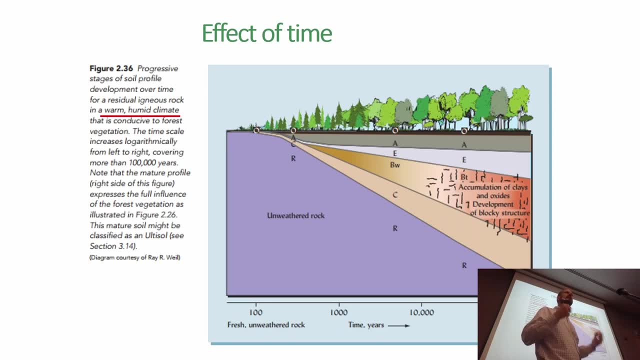 in effect an app, are not lined up so that the soil that comes out of the soil is University of internationally, the. so this by observing in the very表 a and what you can get from the nature of the in Removal. if you have another image project, you can take this next film. 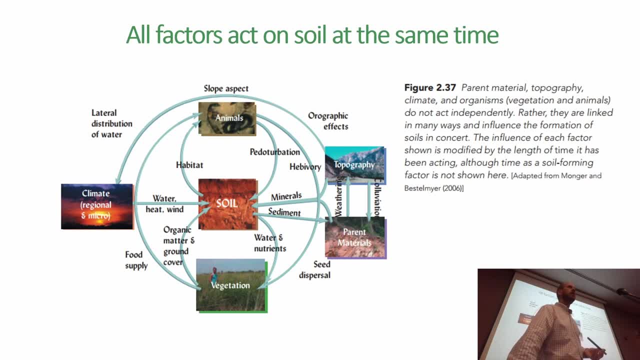 film非 ن ز to check it in. give a little time to see the media process and then you're ready. the next find ofمل time and blend it. as you can see, it takes a little bit more time to blend so觉 and strips and GG around a. 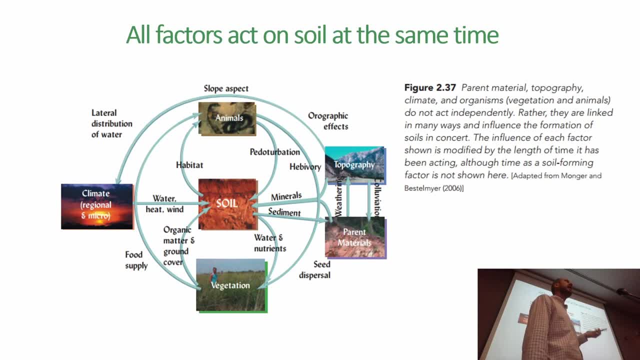 slide here is just to highlight that things are linked together. we are trying to make those links. so topography and climate are changed. if you go up in the mountains, it's colder, there's less temperature, down is hotter. if you go up in the mountains, maybe you have more condensation. so 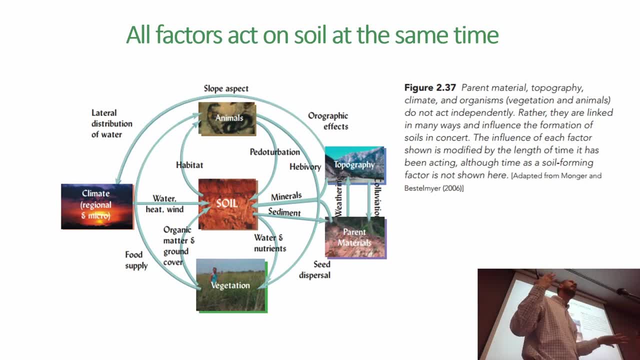 there is a difference between the climate, a relationship between climate and relief. yeah, parent materials also. if you are in the different parts of the topography, you have different parent materials. you have in situ soils formed from the bedrocks, colluvial materials, alluvial materials, vegetation- also related to topography, to climate. so 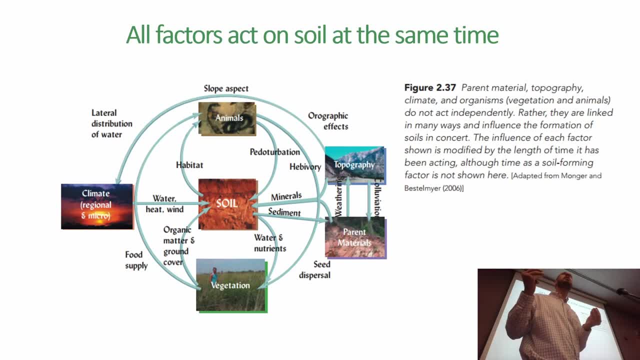 all of that is not is not easy to isolate one effect from the other? yeah, we can try to isolate what is the sequence of parent materials, the sequence of topography, the sequence of vegetation, sequence of climate, but most of the time you cannot separate. yeah, it's not easy to. 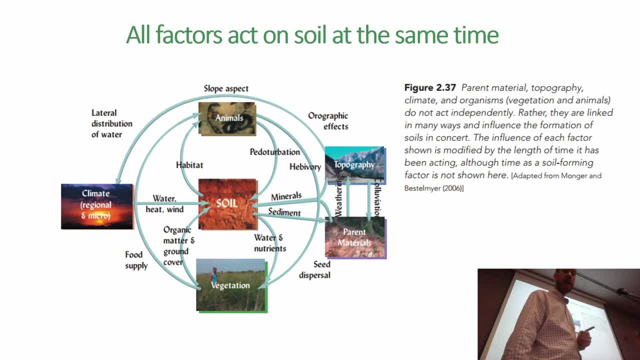 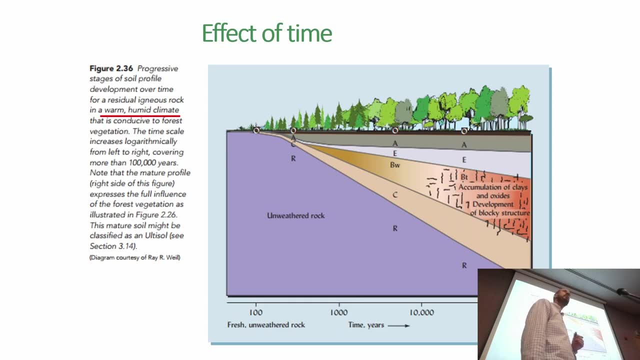 separate the fact of the time. in some places you can separate. yeah, this is called a chrono sequence. yeah, some places you have chrono sequences that are naturally formed. one example is glaciers. glaciers are sometimes retreating back there. you know melting and they're retreating and that retreat has a steady pace. the oldest material brought from the glacier maybe has, you know, 10,000. 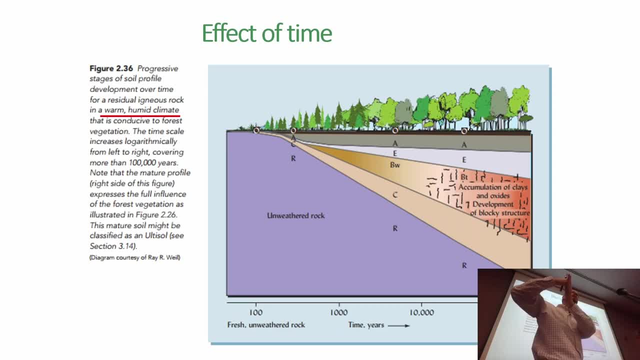 years, the youngest one will have a thousand years or something like that, and then in between you have a difference of time formation. at some point, the glacier starting started retreating an uncovered material at different times. so if you go there and sample, you have a gradient of time actually. 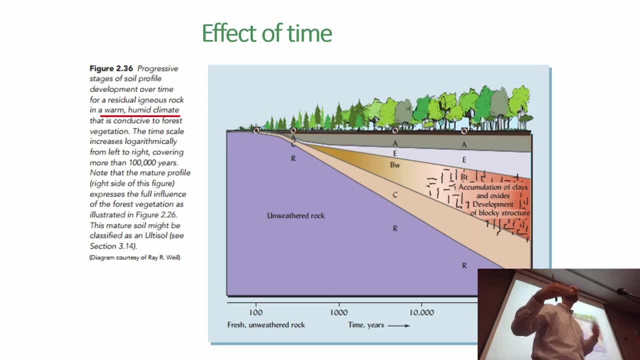 how much, how long those materials were exposed for the formation under the same conditions. they have the similar conditions. only thing was time is different. the effect of time sometimes can be observed in coastal dunes. in australia there is a one of one formation that is. every time you have an earthquake a lot of alluvial material goes into the ocean. 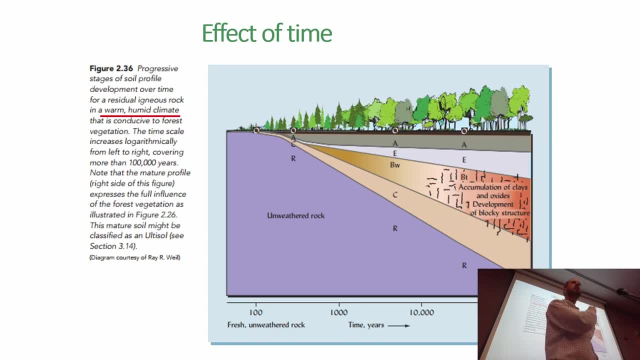 the river brings all the rocks coming from the cacarius rocks goes into the ocean. the ocean brings them back back into the coast and form a dune formation. so over time you have a new dune, another dune. the parent material is the same, so it's just forming layers and 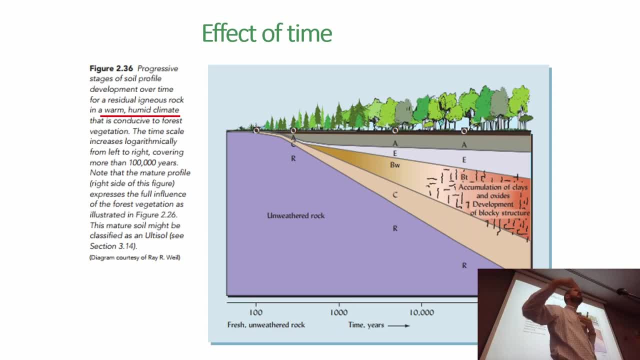 layers and layers of new coastal dunes which are deposited over the coast of the ocean over time. so if you look at this- the same parent material that are deposited in different time scales, and what happened to that soil- you can see the effect of time on that. so this is called a. 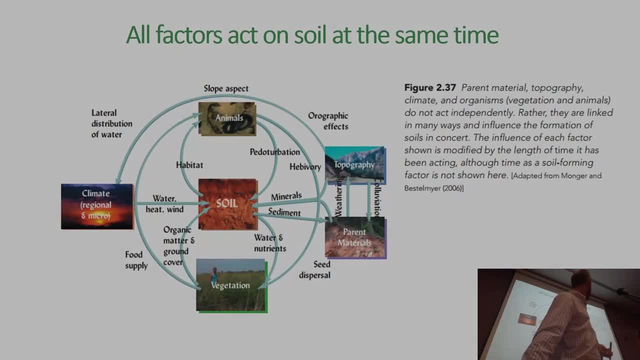 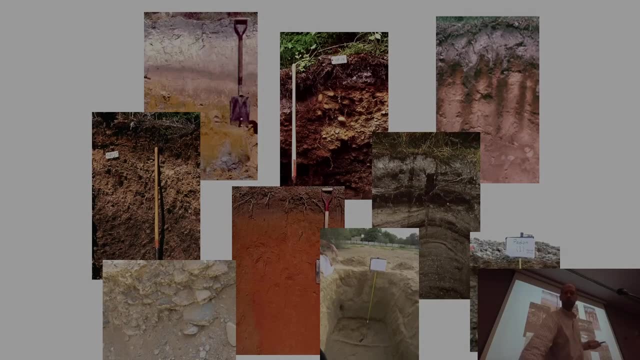 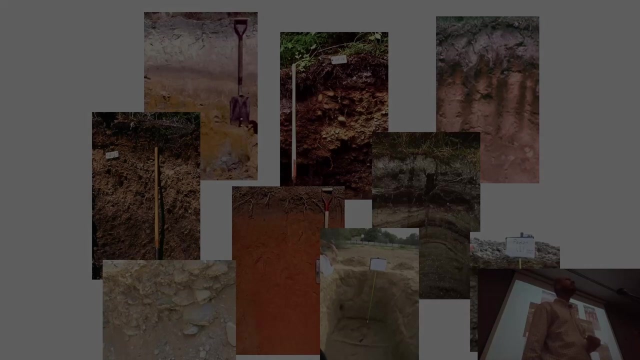 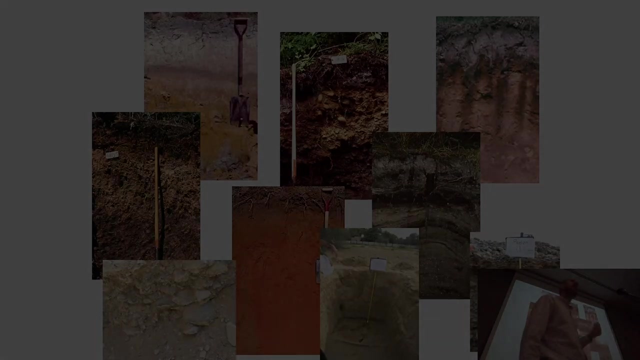 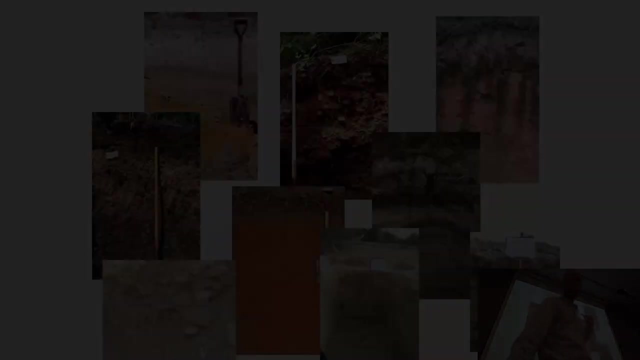 chrono sequence, yeah, chrono sequence. all the others you try to isolate, but they're very hard to separate from each other. yeah, and thanks to this complexity of interactions is that we have the increased vulnerability, ie the pathogen and the kid, but by increasing the density of dynamos it has increased, and the density and beauty of different soil profiles. if you go around the globe, thousands and thousands of different types of soils can be identified, and all of this diversity of soils and their unique properties, or a consequence of these interactions that you see here. that was for today. you.